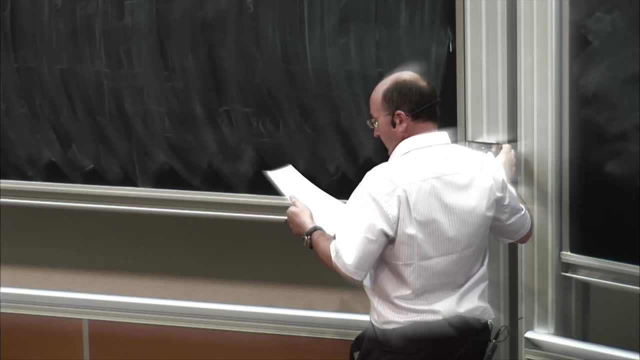 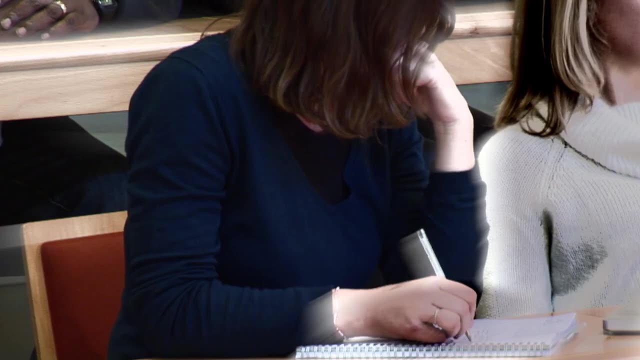 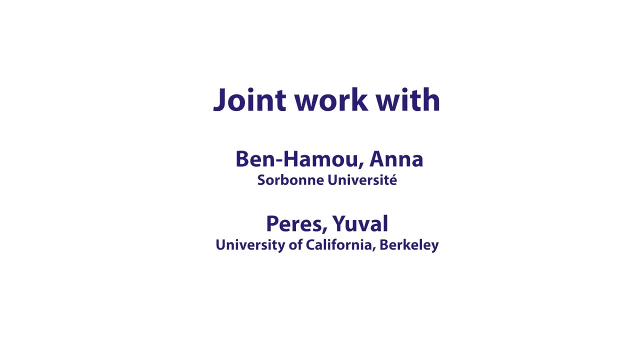 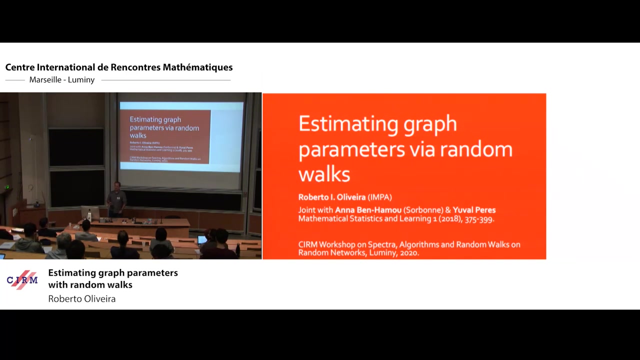 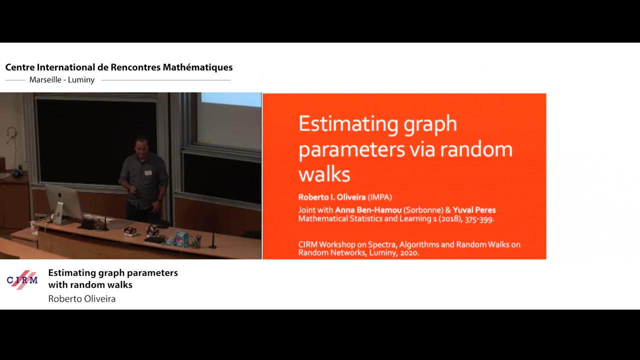 Thank you very much to all of you for being here. Thanks a lot to the organizers for organizing this very nice meeting. It's a pleasure to be here. I was chatting with some people this morning and yesterday and this might be the most on-topic talk of the whole conference. 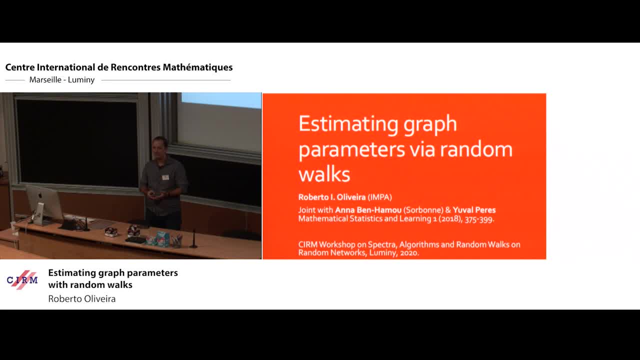 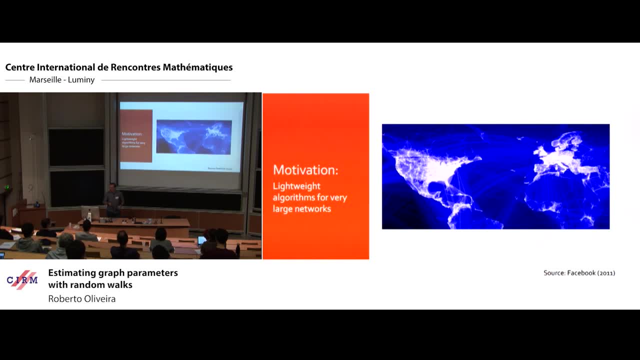 because there are going to be networks, random networks, sometimes random walks are in the title and the spectrum will also show up eventually, Right? so okay, these are just fancy pictures, I guess, but there are people out there, not? 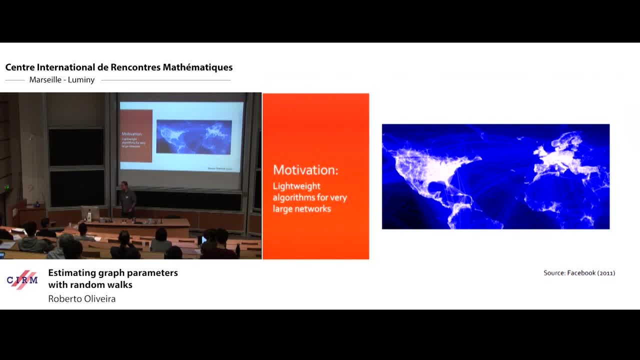 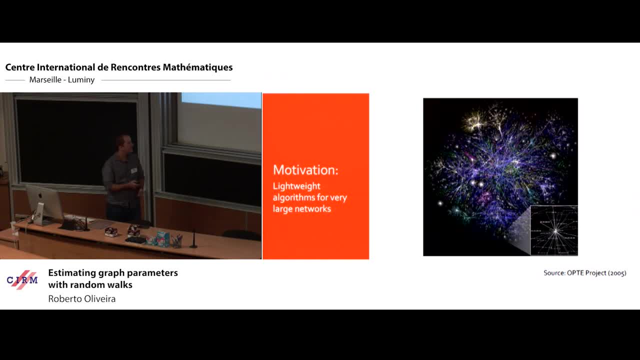 us, but you know people who are practically minded, who worry about developing algorithms for extremely large networks, like you know, Facebook, or this is the physical Internet. I mean, these pictures are old and actually, if you look at the current versions, they're. 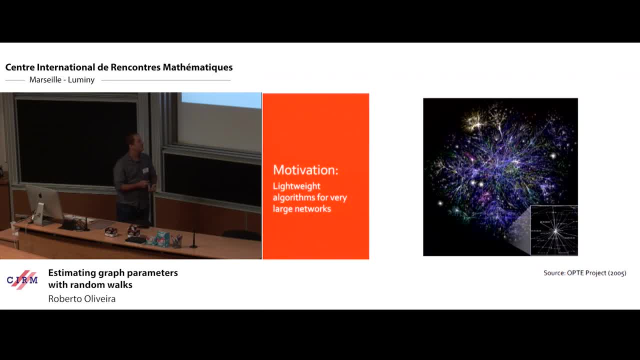 kind of ugly, because they're so dense that you can't really see much. right? This is very nice, but it's from 2005.. The 2018 version is messy and well a lot less pretty than this one. So, people, we have these massive networks and we want to do things with them. 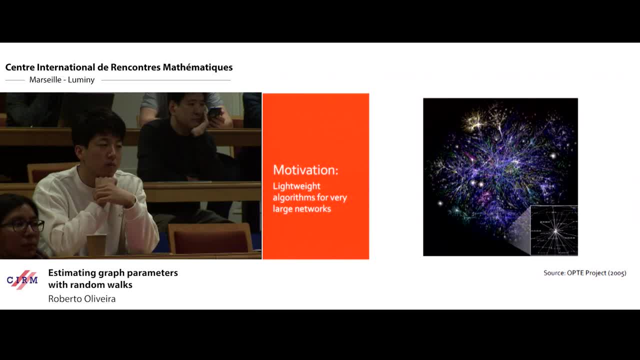 I mean, if you want to do something with them, you have to do something with them. Even simple things like saying: you know, suppose someone gives you access to Facebook servers and you want to count the number of users, right? What are you going to do? download? 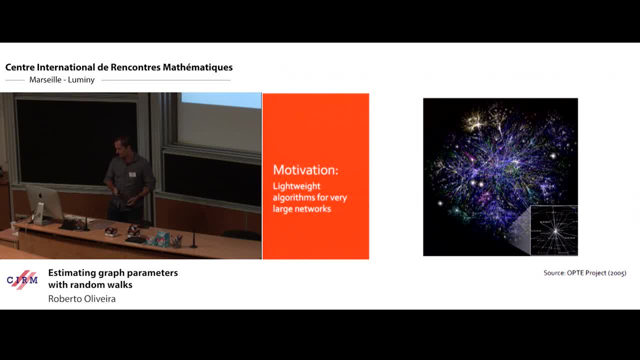 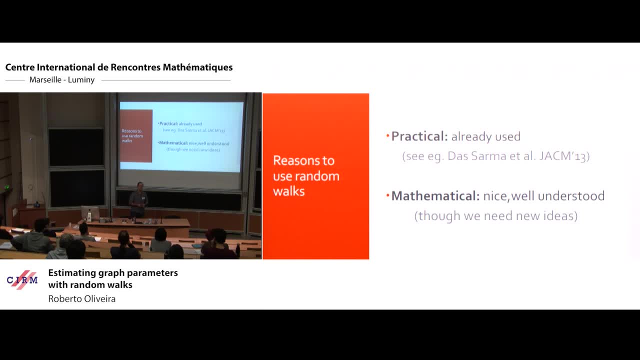 the entire graph to your notebook, or I mean. that's not going to work right, So, and we're going to be looking then at random walk-based algorithms, algorithms that use perhaps several random walks on the same graph to say things about the graph and it's made the number. 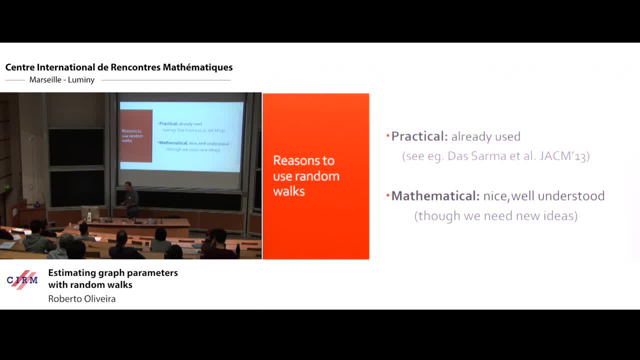 of vertices or the number of edges and the mixing time. those are going to be the three parameters We're looking at, and there are perhaps two reasons to use random walks. One of them is that they are already used by these practically minded people, So it's people actually write. 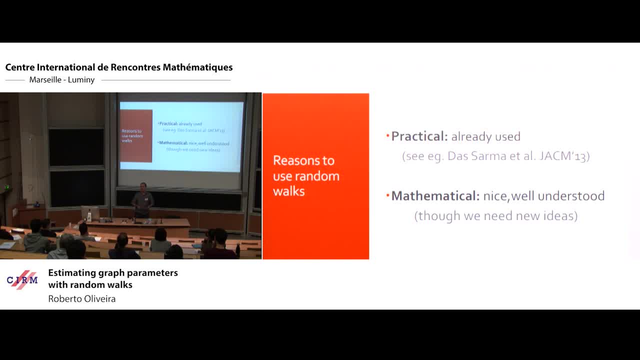 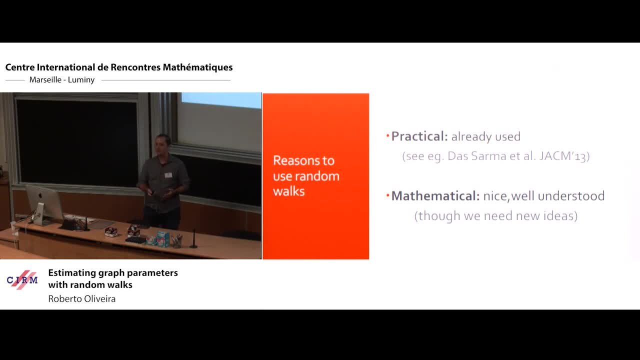 papers about how to implement random walks in distributed systems or large networks, And of course, we know a lot mathematically about random walks, so maybe we can expect to get sharp results in the problems they're going to be looking at. right, So we can. 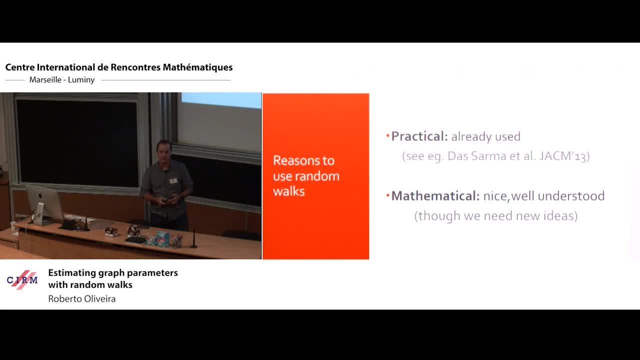 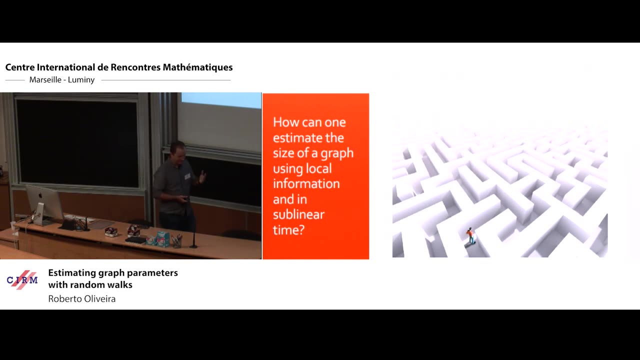 maybe look at- and we're going to be saying a few things about the optimal time, complexity or figuring out a good estimate for the number of vertices in the graph, with high probability So, and perhaps I mean, you know, there's kind of the corporate motivation for doing. 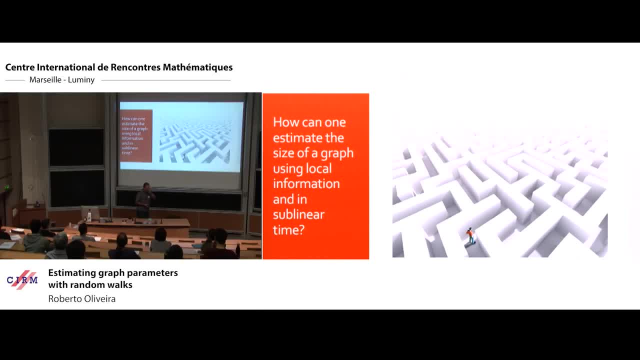 these things right, The practical motivation, but for, maybe, for a mathematician, this is nicer, right. So it's basically the question that got us thinking: is that you're doing this local process in a graph, right? And perhaps a few local processes, a few random? 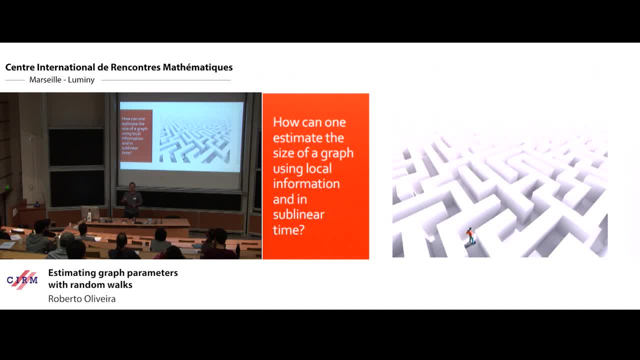 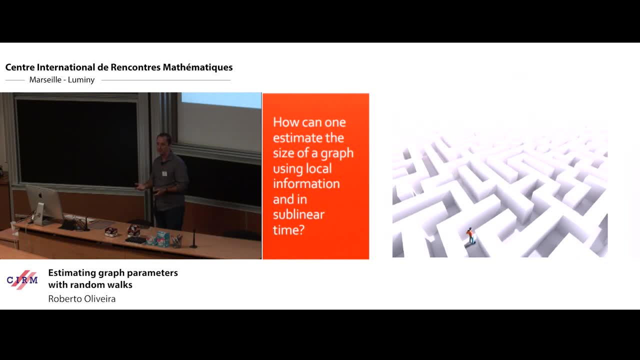 walks, And how do you extrapolate information from that little knowledge you have of the graph along the random walks to say something about the entire network? Is that even possible? right, That's, I mean. it's certainly the most interesting case is when you're able. 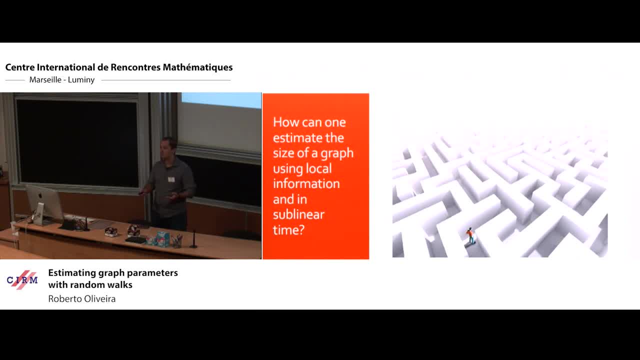 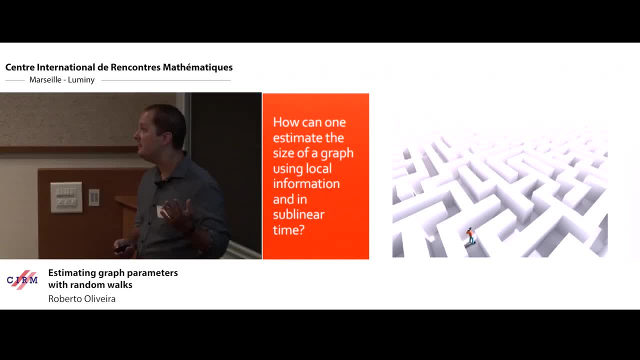 to do it before you've had time to visit a positive proportion of the vertices, right? Otherwise it gets a bit simpler. But of course, when you put the problem like this, it's not clear what you can do, what we're gonna see. we can estimate these things. 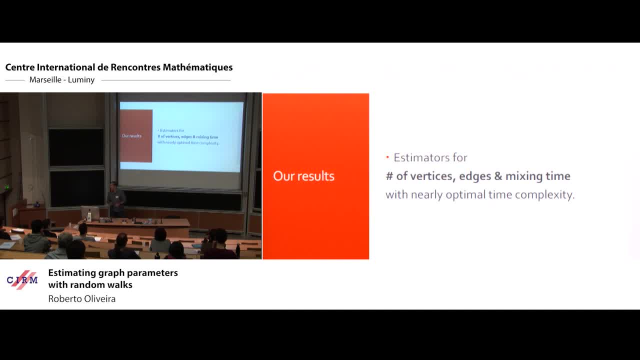 with nearly optimal time complexity, but you have to bear with me so that I can explain in what sense we can estimate right So there, so okay, let's just start with notation. I guess everybody in here knows what a graph is. 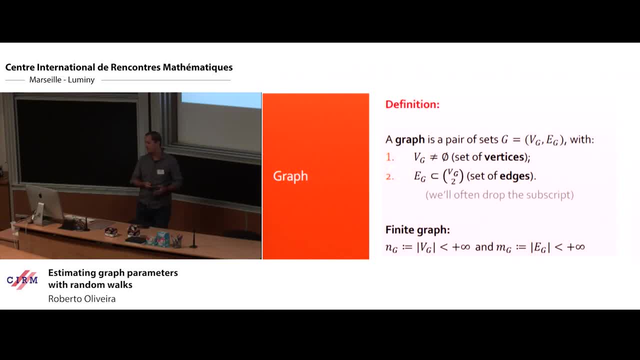 and n is always the number of vertices, m is the number of edges. The graphs are undirected, they have no self loops And I mean this is more notation. you know, neighbors, degree, blah, blah, blah, And I'm gonna be looking always at lazy random walk. 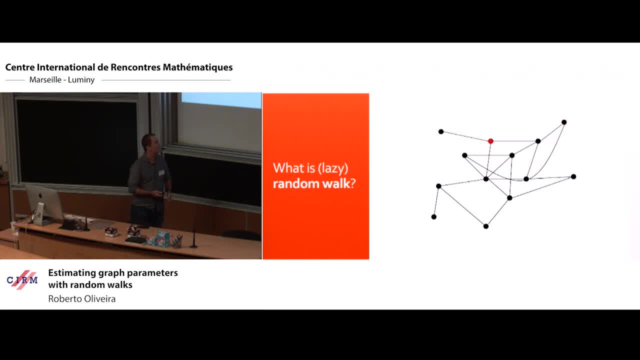 for technical reasons. Well, okay, the technical reason has to remove the spectrum already. You want the spectrum to be non-negative And lazy. random walk is just. you know this process where you say, put the probability a half and you move to a neighbor with probably one over. 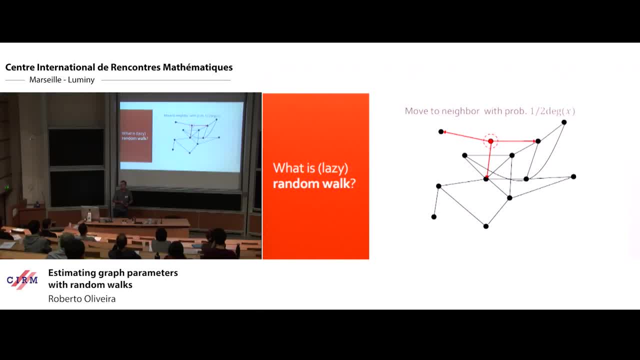 twice the degree, right, Any neighbor has the same probability. And this is just, you know, fancy picture, so maybe okay, And there's even more notation. So we're gonna be looking at several random walks right Indexed by this parameter- i here. 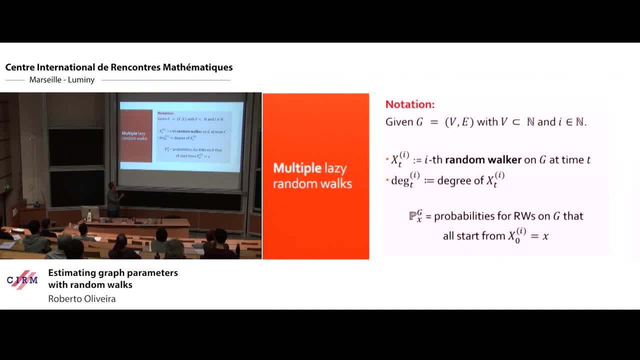 So each one of them is x, sub, t, i, And this guy here is the degree of this vertex, right. So basically, what we see about the red work is what you know: the vertices that have been visited by the random walk and the degrees of those vertices. 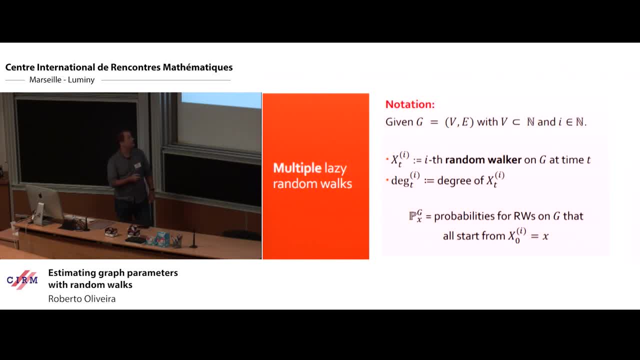 Okay, so we see this And here just saying, I mean I'm gonna use this to say my own graph G and all of my random walk start from point x. In principle, I could allow the random walks to start from different points. 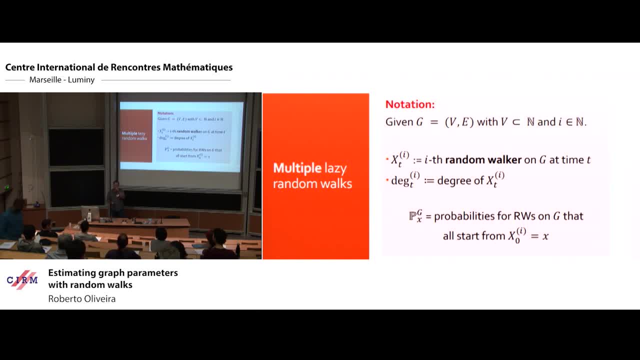 but it really doesn't make to much for the difference in the theory and in this way we get slightly cleaner results. Could think that maybe you know. let me move on. Basically, we can think that this starting vertex is chosen by an adversary and we wanna do as well as possible. 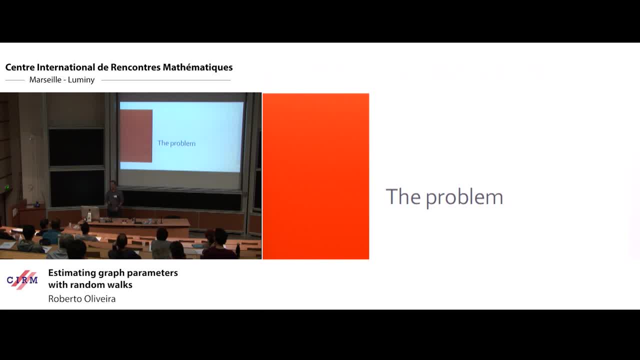 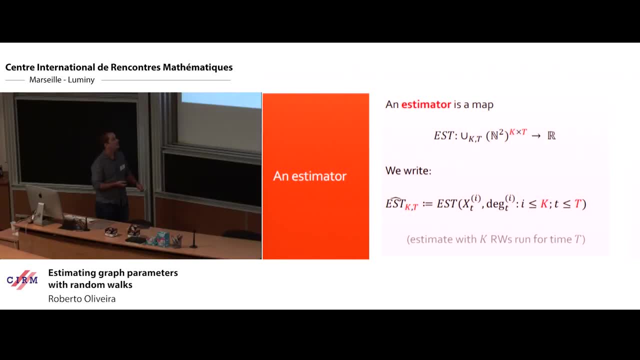 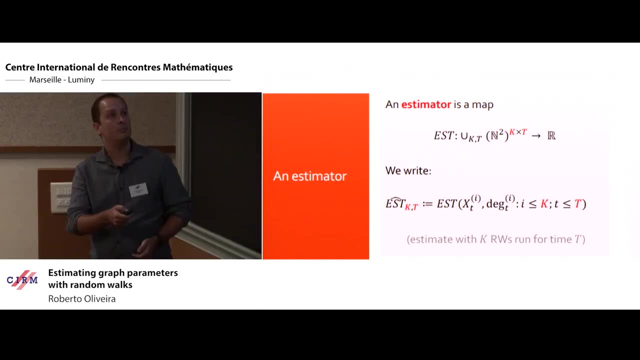 wanna do as well as possible given that restriction. So, okay, we're gonna be estimating things. What's an estimator Here? I'm basically assuming that all graphs I look at have their vertex set contained in natural numbers, So the input to an estimator is just a sequence. 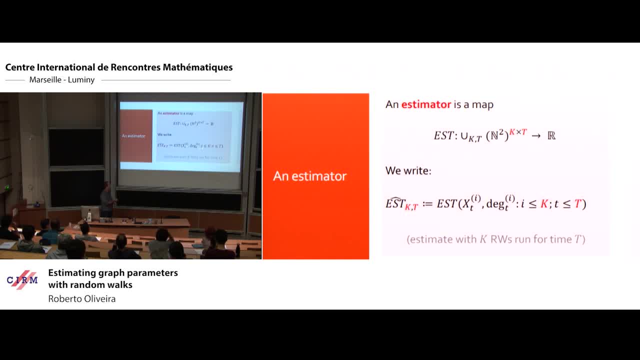 of vertices and degrees seen along the way by the k, random walks by up to a certain time, capital T. And given a family of graphs and say a parameter like the number of vertices of one of these graphs, I wanna prove results of this kind, right. 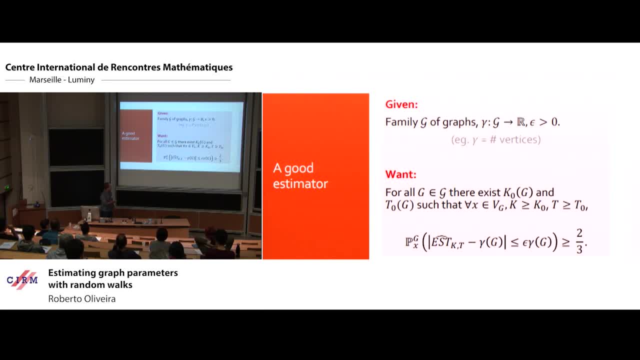 That for any graph in my family there exists a number of random walks in a certain time, such that if I have at least as many random walks and I have at least that much time, then no matter where I start from, I'll get a good estimate. 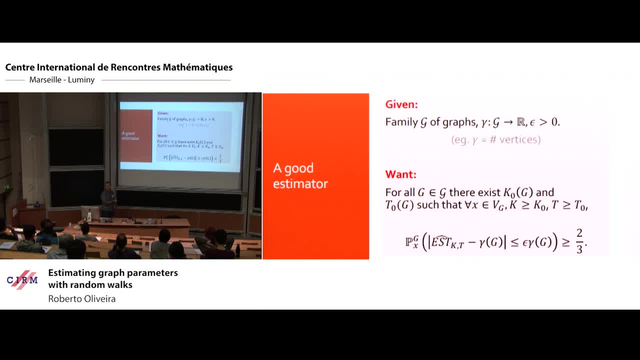 for this parameter with high probability, right? So this is saying that I estimate gamma of g up to a one plus or minus epsilon factor, And I mean so the time complexity is just a total number of random walks, right That you multiply the number of random walks. 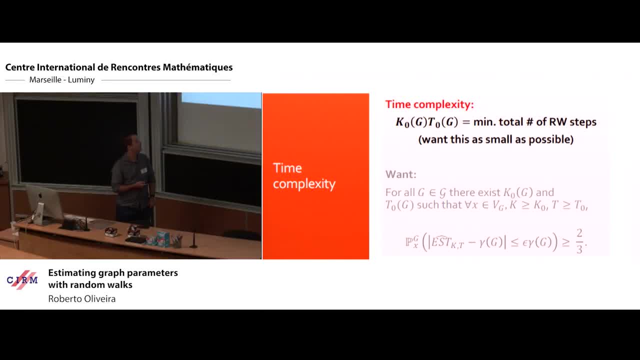 by the time that you use. But I mean- and this is sort of a funny definition, because I'm saying that- I mean, this is not the way we usually do things, perhaps because we're saying: okay, my time complexity is somehow dependent on the graph g. 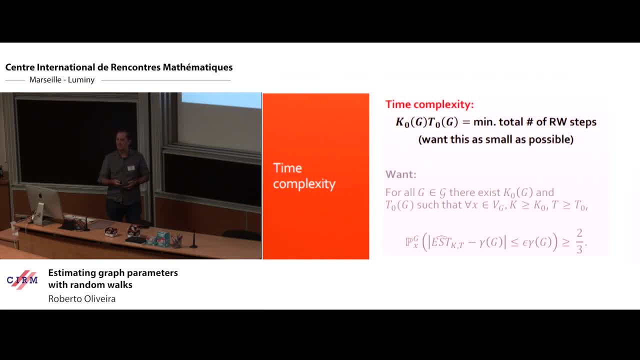 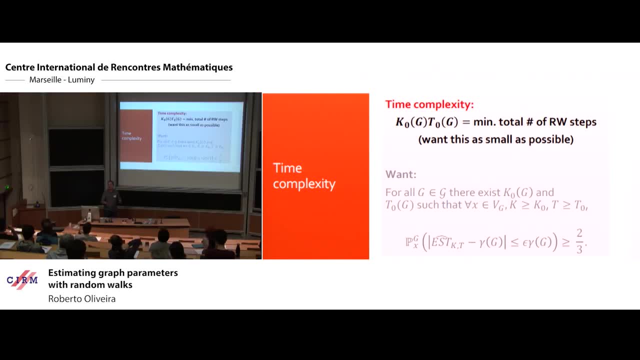 which I really don't know right. So there's something odd about this. So it's saying: okay, I can prove that. perhaps my time complexity square root of the number of vertices. but I don't know the number of vertices. Perhaps that's even the parameter I'm trying to compute. 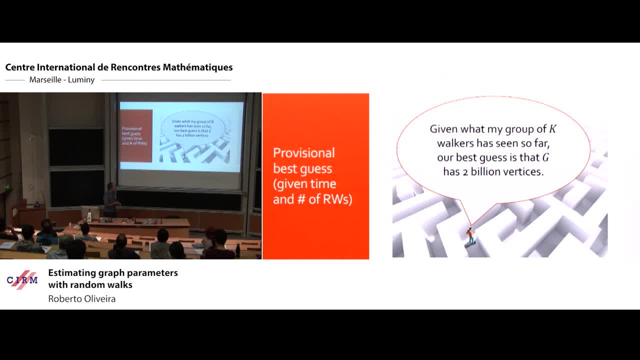 So it might sound like it's a bit funny, but bear with me, But okay. so just to make sure we understand, I mean intuitively- what we're doing is we have these random walks, walking in this, this labyrinth, right? 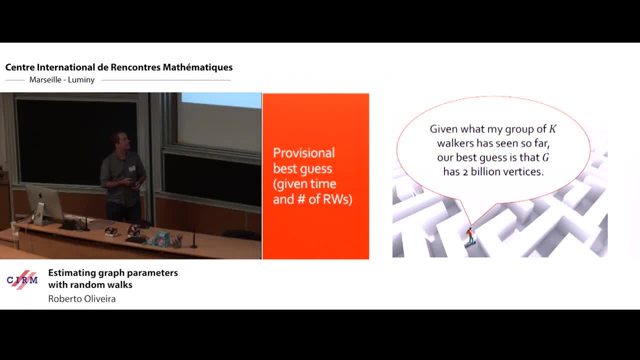 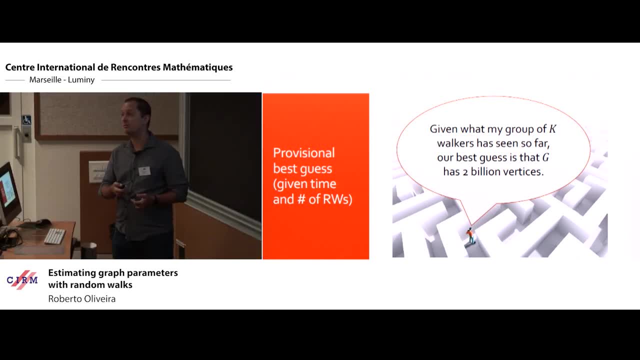 That's the graph And at any given time you can ask what's the best guess they have for, say, the number of vertices in the graph, And that we want this best guess to be right, with k as small as possible and time as small as possible. 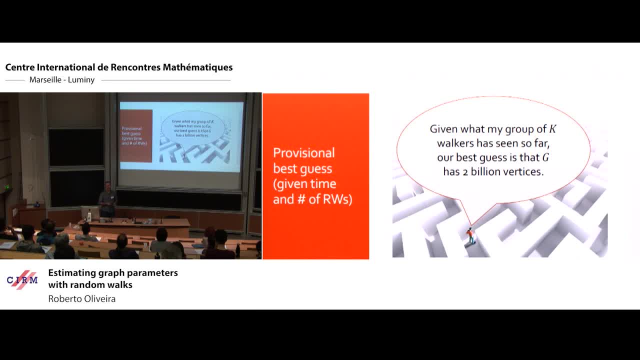 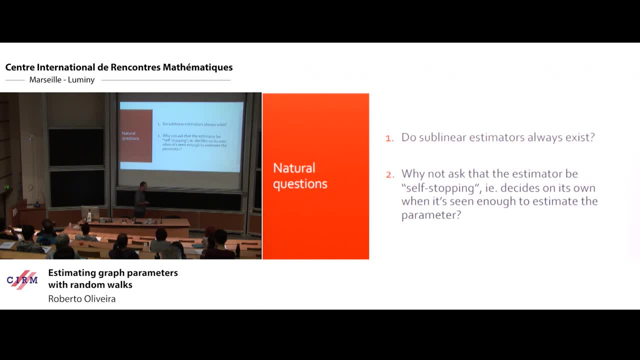 What we want it to be: right, with high probability right, But probably greater than a half. basically, And as I said, the most interesting case is when you have sublinear estimators, right? It's not clear that you can always get sublinear estimators. 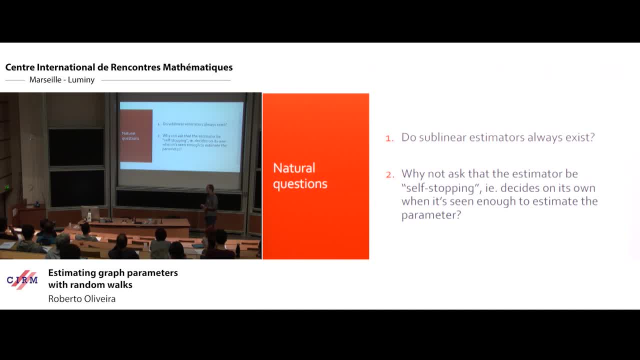 and we're gonna see that, in fact, you cannot always do that. Here's another thing that's perhaps more subtle, right? So one thing that would be really nice if you could get these algorithms to work, but not only that: they work. 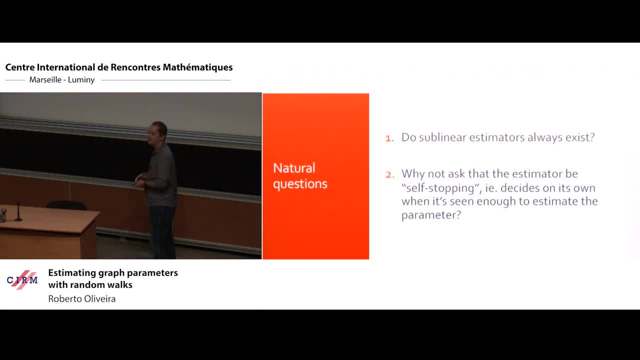 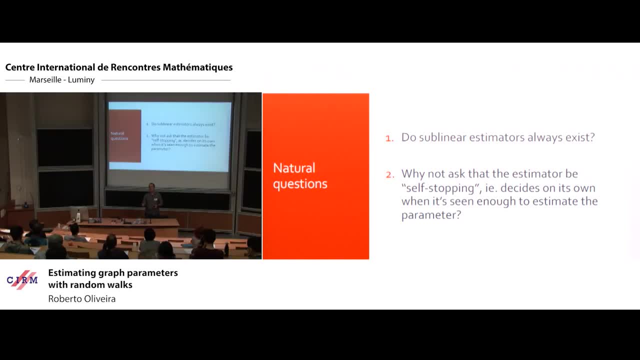 and they decide on their own when they've seen enough of the graph. right. So the random walks start walking around the labyrinth and eventually they decide. now we can stop and give you a good estimate of the size of the graph, with high probability right. 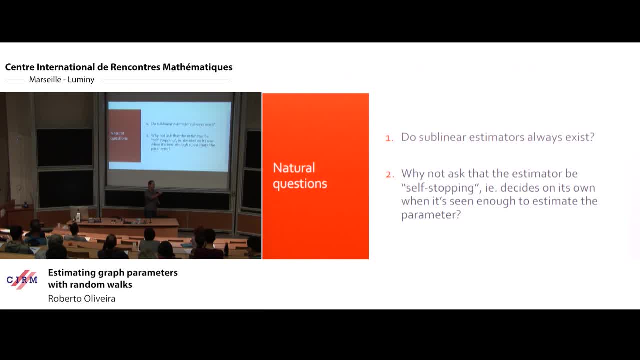 That would be what I call a self-stopping algorithm. That would be what I call a self-stopping algorithm. That would be what I call a self-stopping algorithm: An algorithm that has a stopping time at which it can make a good prediction. 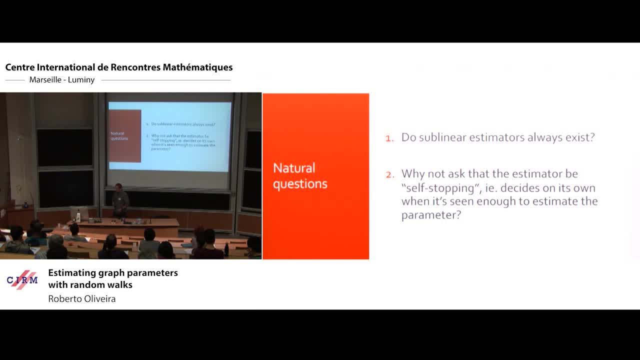 or a good estimate, And but, as we're going to see, these algorithms don't really exist in interesting contexts, So we have to settle for a weaker definition, So okay, so perhaps it's good to start with some examples so that we understand what are the limitations. 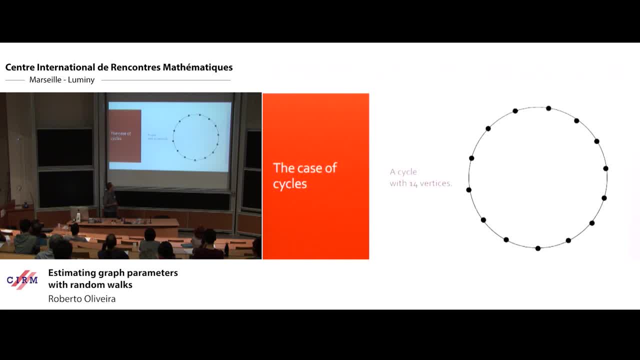 of this problem, right? So let's assume that our family of graphs is just cycles. Cycles are a different number of vertices, right? And how do you figure out the size of the cycle? Well, my claim is that, for a long time, 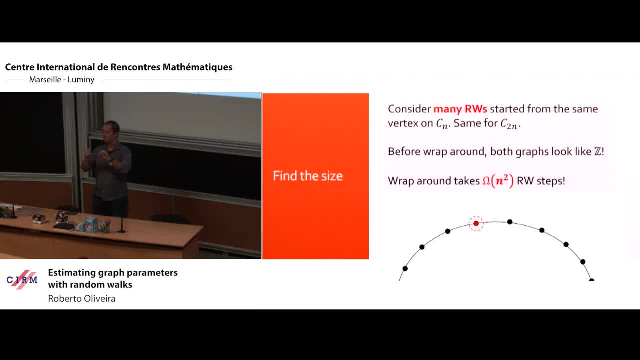 when you walk on a cycle, you don't see anything but a line, right? We know that you need n squared steps to just wrap around the cycle. So if you're walking, if you have random walks on two different cycles, I mean let's say okay. 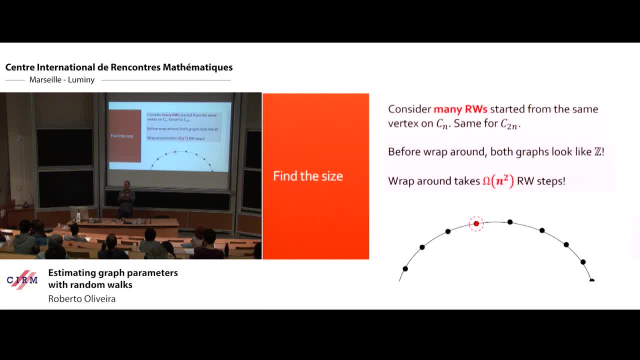 there's a slightly non-obvious fact, which is that if you start k random walks from the same vertex in your graph, the time it takes for one of them to wrap around is still of order n squared, I mean the total time right. 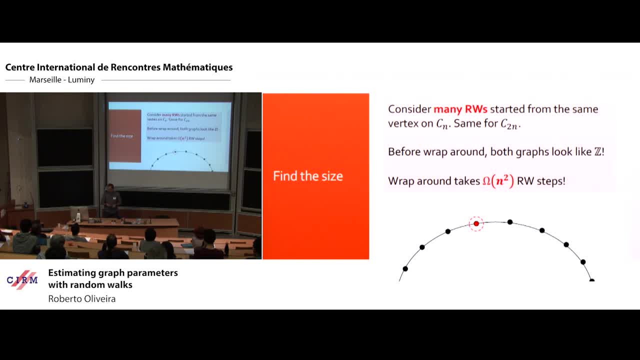 The total number of steps. And well, in some sense you're better off just having one random walk trying to wrap around, Right, so, but okay, so it takes a long time for these random walks to see, to notice, for instance, that the cycle is not the line, right? Okay, so it takes a long time for these random walks to see to notice, for instance, that the cycle is not the line right. Okay, so it takes a long time for these random walks to see to notice that the cycle is not the line right. 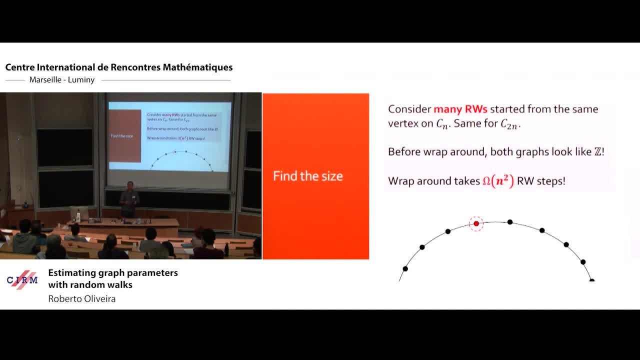 The integers right. So up to that time you can couple random walks, say on a cycle size n and a cycle size two n, so that they see the same thing, Or perhaps to the labels of the vertices. but you can match these. 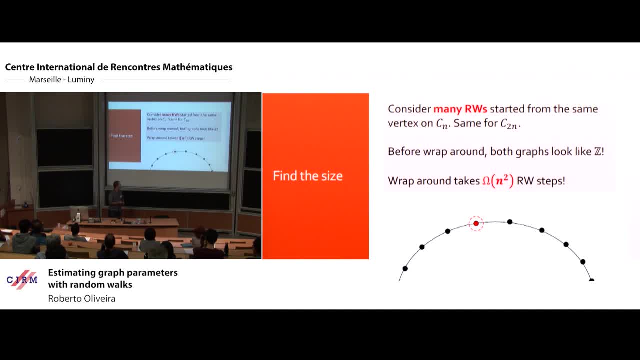 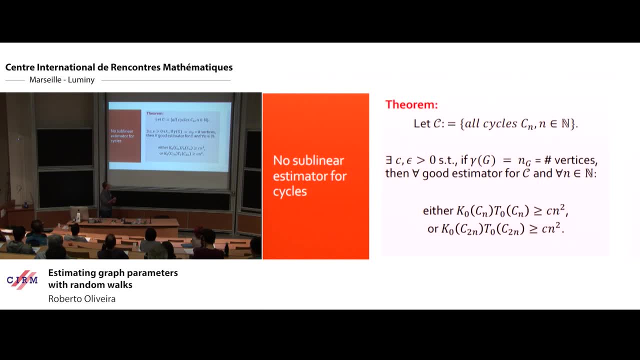 so that you can really tell the graph apart. So okay, this is the first non-trivial theorem that we have in this model. It's slightly non-trivial. perhaps You have this family of cycles, Your parameter's, the number of vertices. 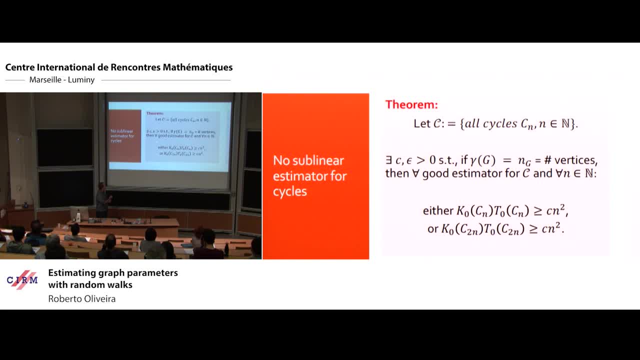 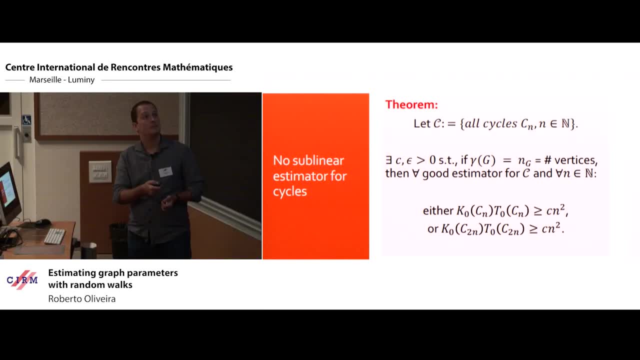 So what this is saying is that for any- oh, I mean- good estimator, this should be, this should be just an estimator that works with probability greater than 2 3rds right, So you can say that either a total number of steps, 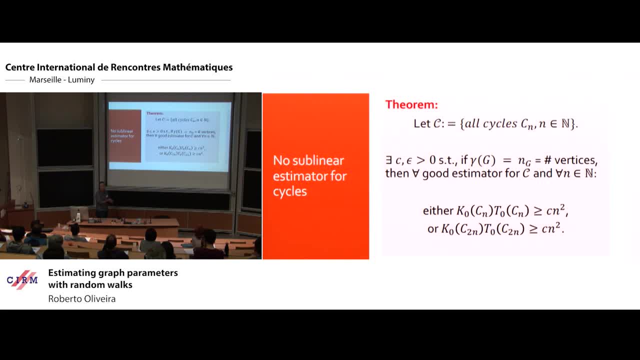 you need to find you need for the cycle size n is greater than n squared with an absolute constant in front, or this holds for the cycle size two, n. Why such an either-or statement? Because I guess my definition allows for an estimator. 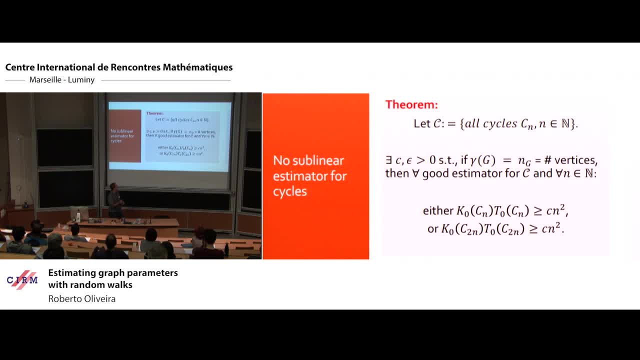 that always outputs n or something like that, right? So basically, this means that? well, among other things, it means that for any estimator to choose, there is gonna be an infinite sequence of values of n, or perhaps half of the integers are gonna be such. 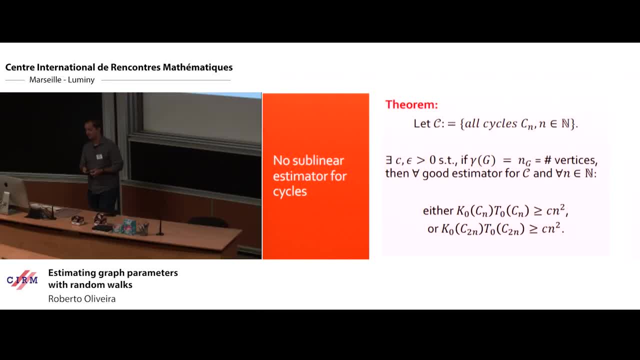 that you need more than n squared steps to figure out the size. So you see, even though we have our weak definition, when you don't have the self-stopping property, this property of stopping time, there's still intrinsic limitations to how well you can do things. 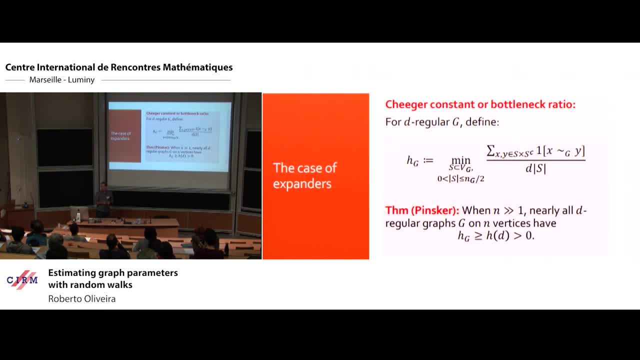 Right, so now let's talk about the case of expansion, In this case, of expanders, right? So maybe people know what an expander is. it's just a graph where, for any subset of the vertices that contains less than half of everything. 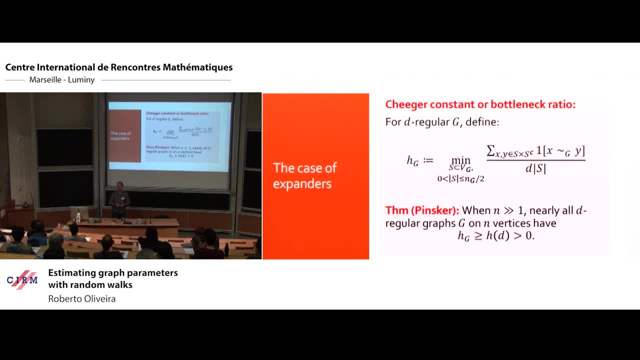 there's a positive proportion of edges going outside that subset right. So the graph is deregular in this case And we know that typically n regular graph- oh I'm sorry, a deregular graph on n vertices is an expander with high probabilities. 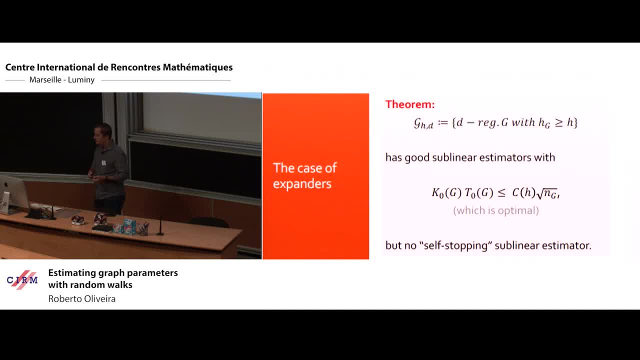 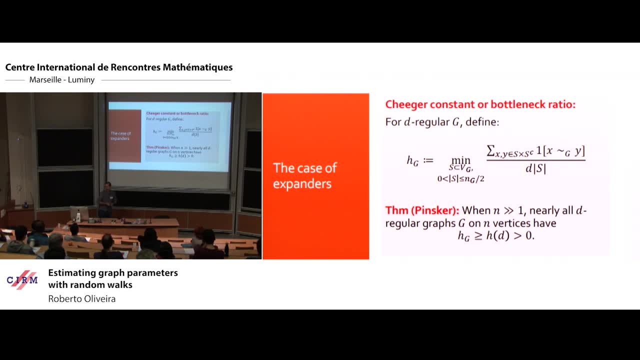 So let's look- okay, that's just to say, I mean, this parameter h sub g is a Cheega constant. It tells you exactly this. it's this bottleneck ratio. And let's look then at a class of deregular graphs. 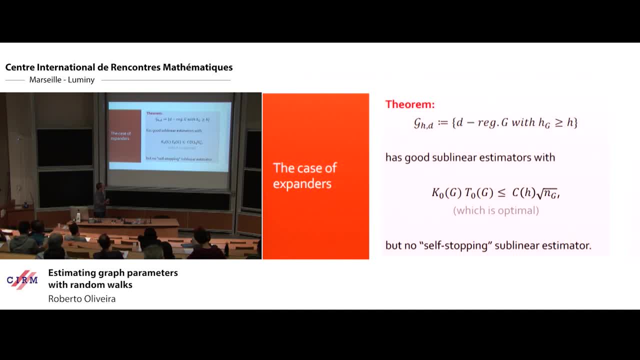 with h sub g greater than h. We're gonna see later that we have good estimators for this class. I mean, we can get estimators where this holds, which maybe should remind you of the birthday paradox or something like that- And but there are no self-stopping properties. 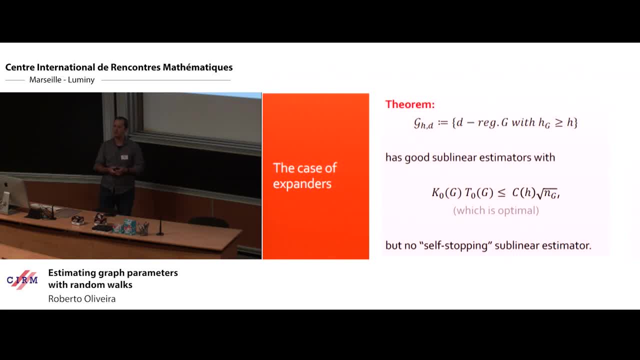 There are no self-stopping sub-linear estimators for this class. Remember that self-stopping is an estimator that has a stopping time and says: okay, right now I can stop and make a good estimate of the size of the graph, Okay, so why is there no sub-linear self-stopping estimator? 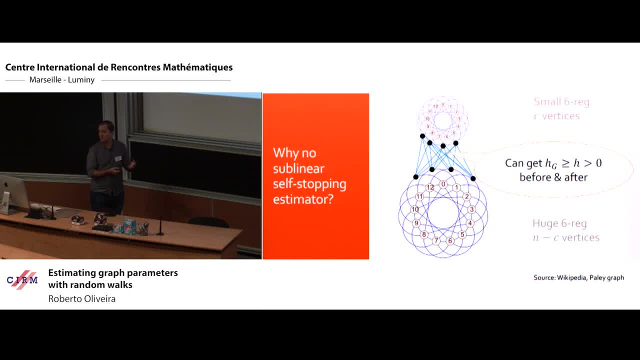 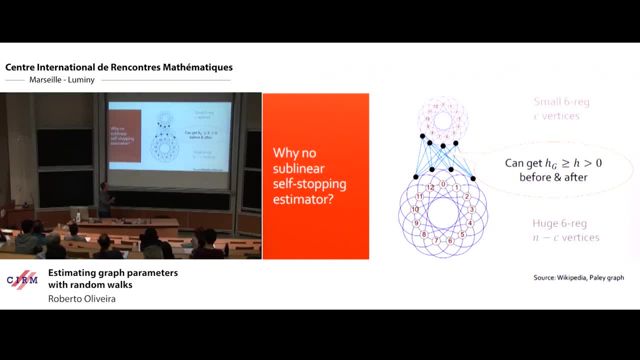 Assume that there is such an estimator and that works for a certain value of c and c I'm gonna think of as a constant right. So we're probably 2, 3rds. this guy walks. he walks on a small fraction of the vertices here. 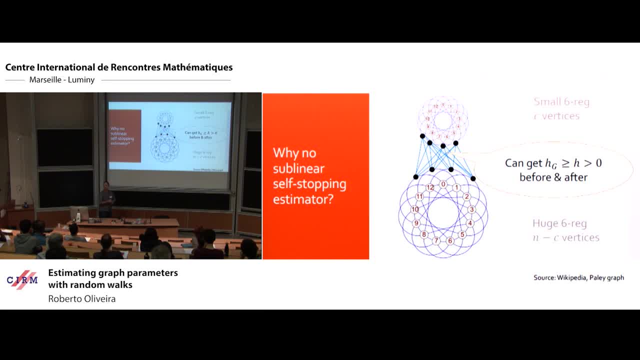 and decides. well, I've seen enough of the graph to say that its size is, I don't know, c up to one plus or minus epsilon, right. Well, what you can do is you can always glue such a graph to a much, much larger graph. 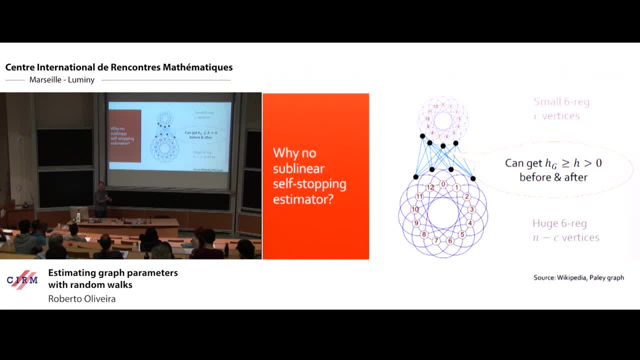 While keeping it as an expander. perhaps you're gonna lose something in the Cheega constant perhaps, But if you make this- well, if this is a constant and there's some very large number- you can get things to work out. 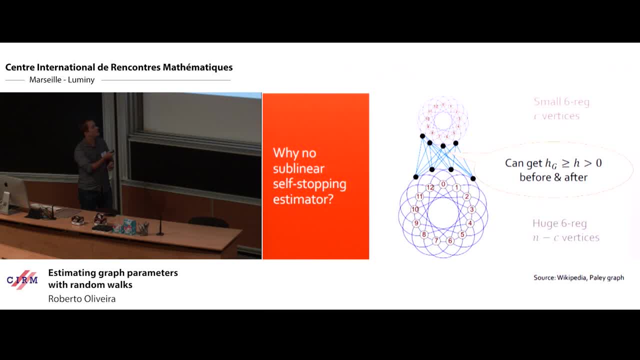 But then clearly, if random walk or the k random walks don't have time to visit one of these vertices here, they won't have time to figure out that perhaps you're in this much larger graph, And then it's clear that you have a problem, right. 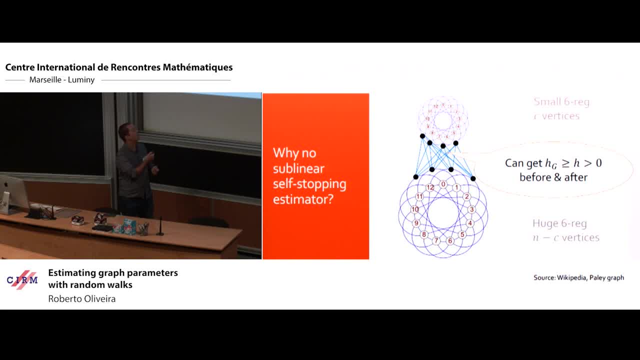 So if the random walk, the random walks- decide in some linear time that they've seen enough, they might be stuck in here and not notice that there's a world out there, so to speak. So there are limitations. I mean, you can make this. 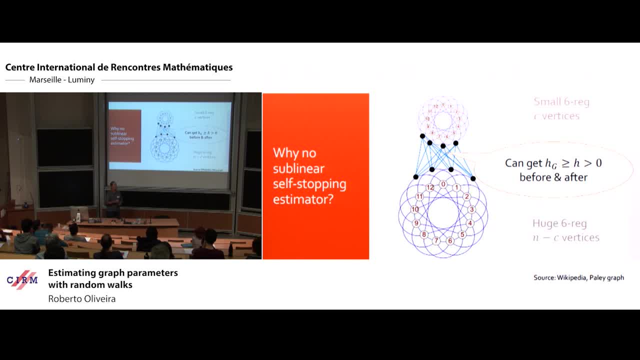 you can make variants of this example where perhaps this: okay, maybe you say I don't care about any constant number of vertices, maybe I care about kind of a growing sequence of values of c, and then maybe you can look, you can get such an example with the Cheega constant. 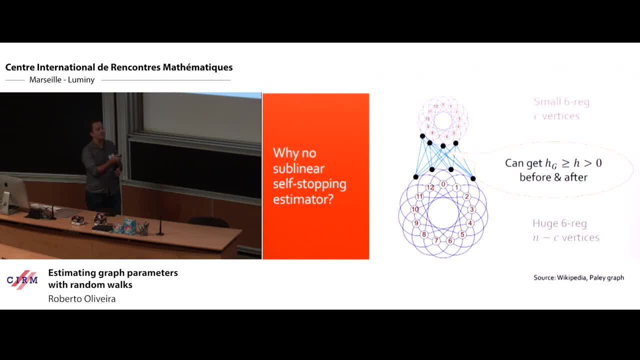 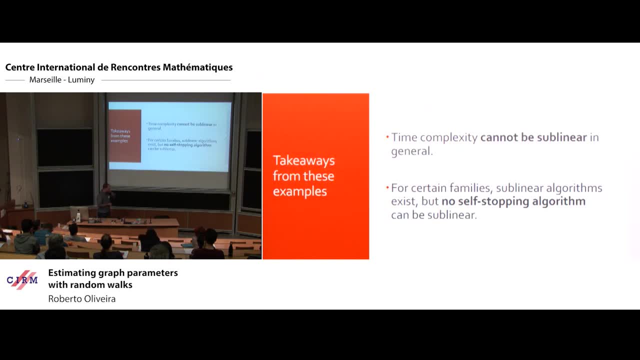 being any function that goes slowly to zero, even if you allow this c to grow somehow. So, yeah, so the complexity. so what we've learned? okay, from cycles? we learned that we cannot get sublinear complexity in general, So we need some assumption on the graph. 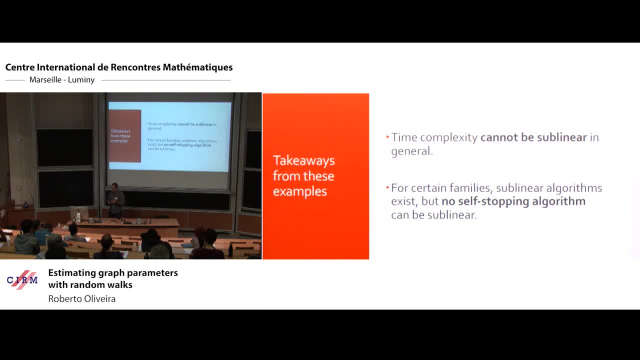 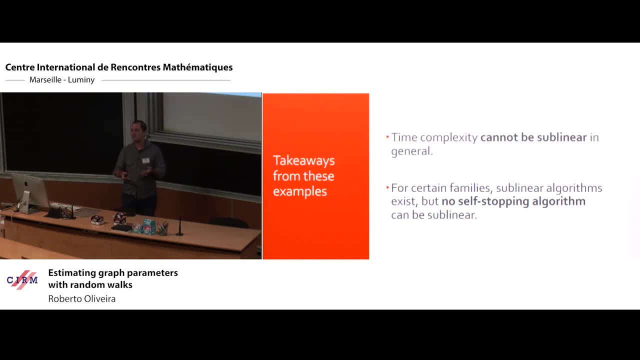 to get sublinear complexity, And there are families like expanders, as we're going to see. there are sublinear algorithms for them, but there are no self-stopping sublinear algorithms, And so we're gonna just decide to not look at self-stopping. 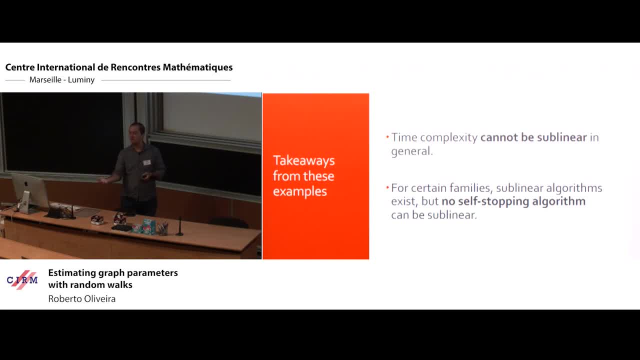 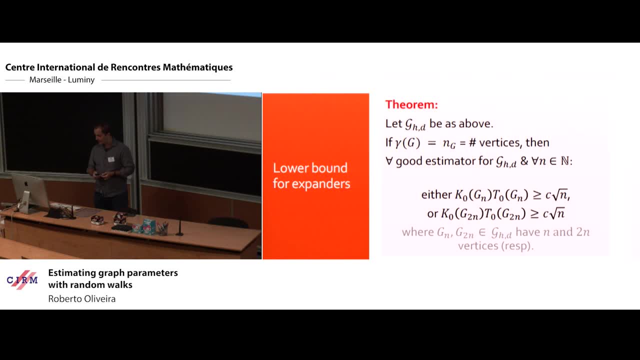 though we do have a few results saying that perhaps, if you know the number of edges, you can compute the mixing time by a self-stopping algorithm, and vice versa. So okay, let me give you. let me give you another lower bound right. 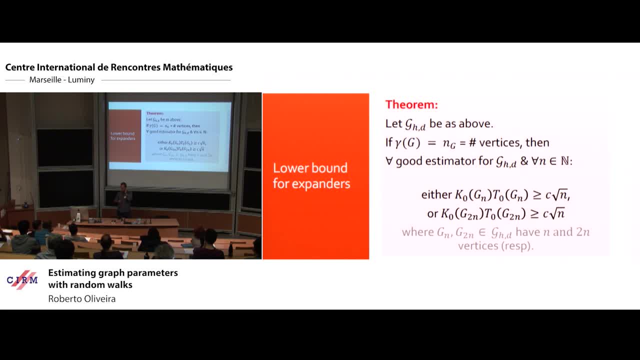 I gave a lower bound for cycles. Let me show you that- and this is very important for the rest of the talk. Let me show you that for expanders there is a square root of n, lower bound. So I claim that there is an upper bound of square root of n. 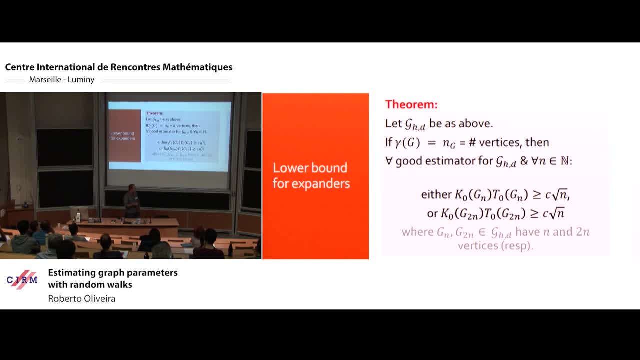 I haven't shown you why, that's true, but we'll get to that, And now. but now I'm gonna show you the lower bound. And the lower bound is based on something we saw yesterday. in whose talk was it? in Who? I mean? someone talked about the configuration model. 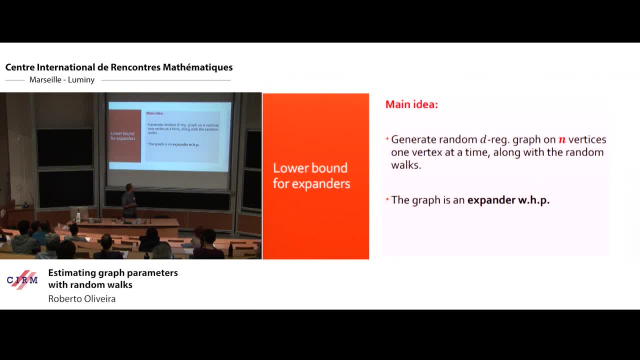 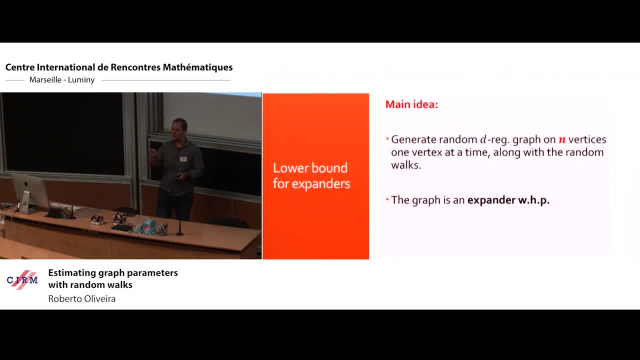 I can't remember who it was, But it's basically so. what we're going to do in order to prove the lower bound is to generate the random graph and the random walk, or the random walks, if you want, at the same time. 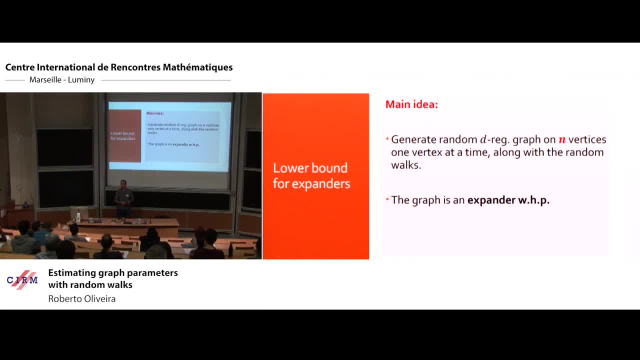 So I'm gonna pretend there's just one single random walk because it's easier to explain. but the same argument works for k. random walks started from the same vertex And we're gonna generate the random walk and the random graph we generate by the configuration model, right? 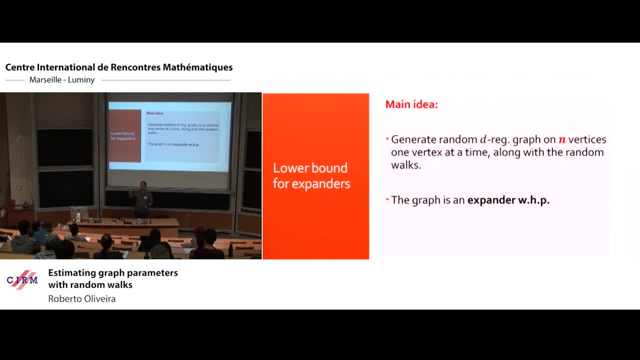 Which is the same way you take, in this case, d half edges representing each vertex, and you take a random matching of the d half edges And but I mean you can't generate this matching sequentially, right? So you take one half edge and you ask: 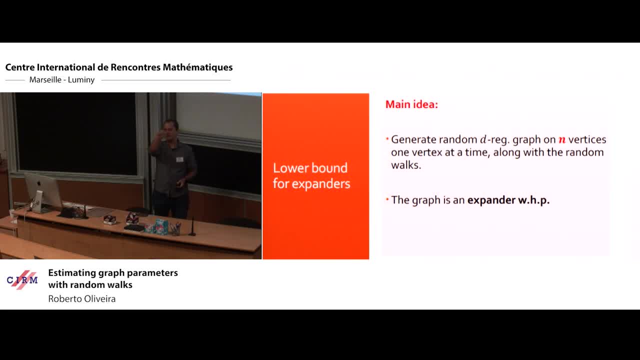 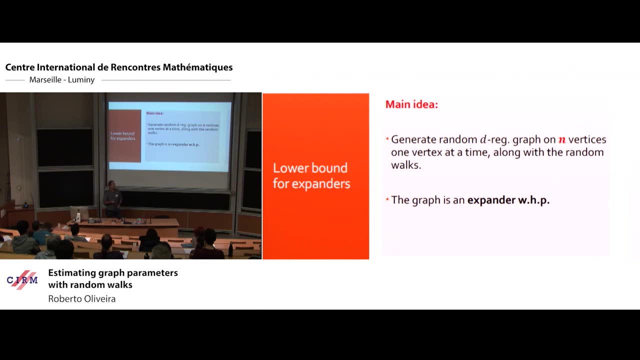 who's this guy matched with. And you go there And then you can in any fashion. if you query for who is the guy that's matched with this guy, you get the same model, the same configuration model. So what we're going to do, essentially, 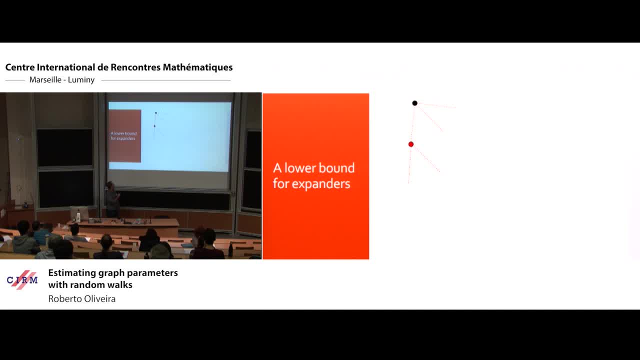 is we're gonna query just for the guy I mean, we have to jump somewhere random walk, has to jump somewhere here. So it queries out who's the first neighbor of this guy, And then it sees something and there are these. 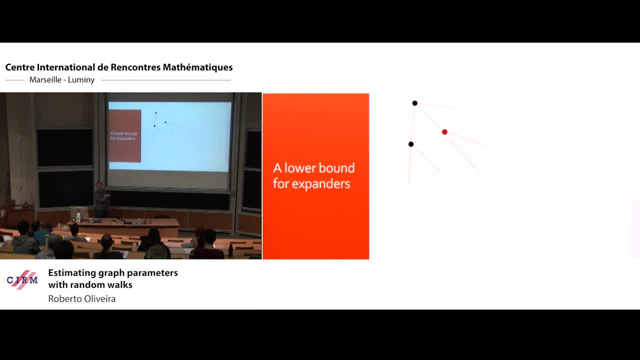 yeah, then it goes back, perhaps, And then it goes somewhere else. so we query for another vertex, And then then we go back, and then we go somewhere else And the chips keep revealing the graph, little by little, right? Well, we do it for a long time. 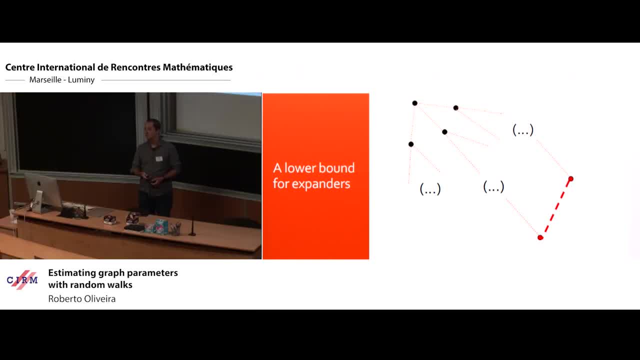 and eventually you're gonna find a cycle. But how long does it take for you to find a cycle right? So it takes you square root of N steps by some kind of Roth current of argument. What happens before then is that you can really couple. 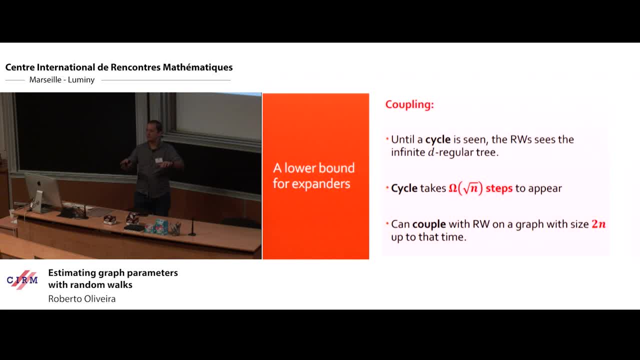 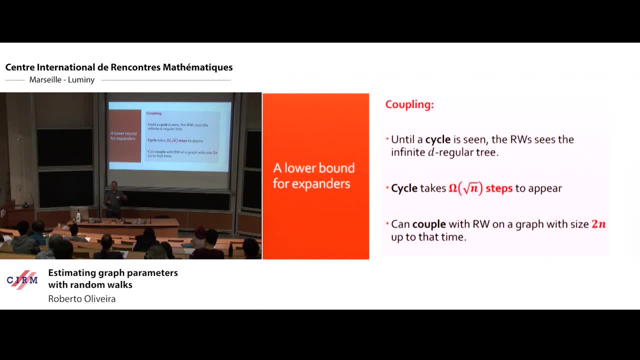 this process on a random graph of size n. so we generate this particular process on the random graph with size N with the similar process in a random graph of size two n, and you won't be able to tell the difference between the two until the first cycle appears in the graph of size n. 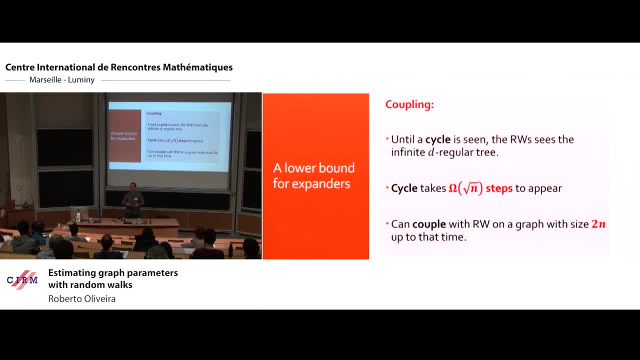 Or you could say that before the first cycle appears, you don't know whether you're walking on an expander or on an infinite deregulatory, And once you put it that way, it's sort of clear that you can't really say anything about the size of the graph before times squared of n. 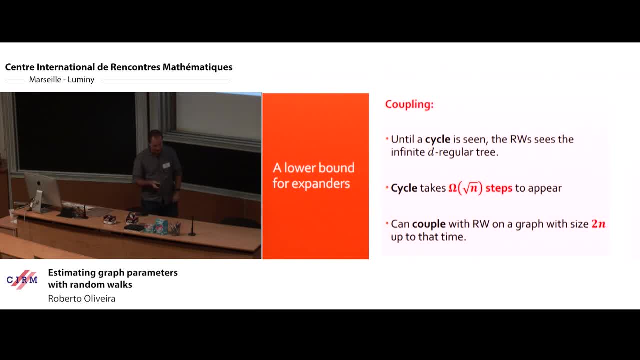 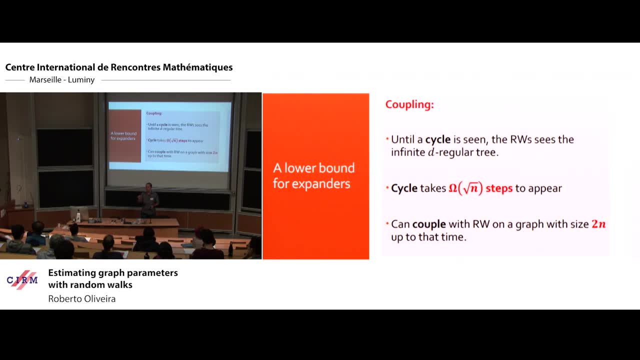 Maybe I should mention- because I'm gonna be talking about that at the end of the talk- is that this is in some sense, a very general lower bound, So you can have algorithms that are more general than ours that we call random walks or restarts. 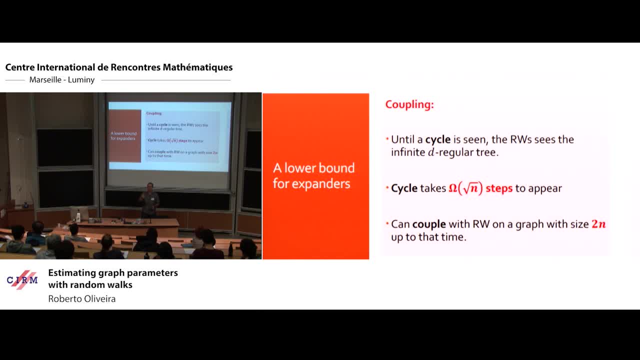 which are just. you have one random walk trajectory, but you can press a reset button at any time and send it back to the starting point. You can have any sort of growth model where you're growing the set of vertices that you have seen by adding a vertex. 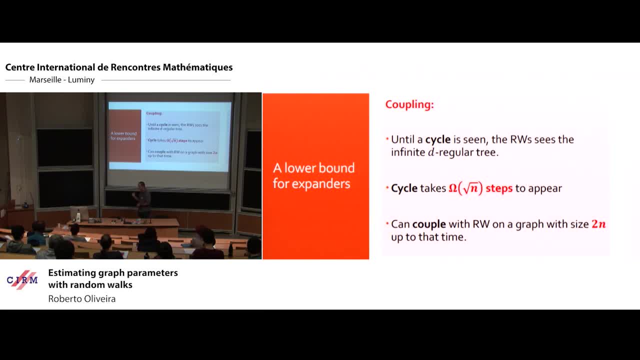 that's at the boundary of the current set For any such model. you get this, So it's lower bound. I'm not being very precise here, but hopefully you get the idea Right. so, okay, now we have at least two lower bounds. 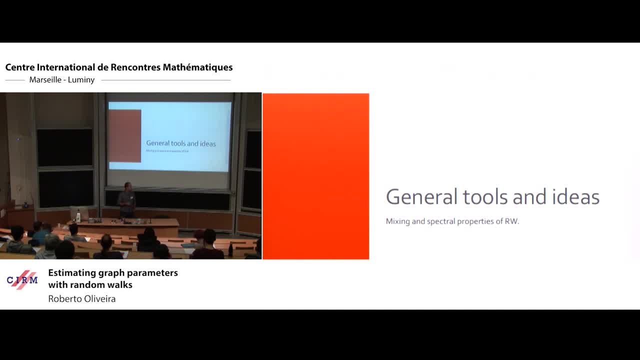 and let me perhaps jump ahead a little bit and say that all of our lower bounds are essentially gonna be based on this expander example. But now we should say something about what we can do. I mean the positive results, right And well, I mean. so that's sort of 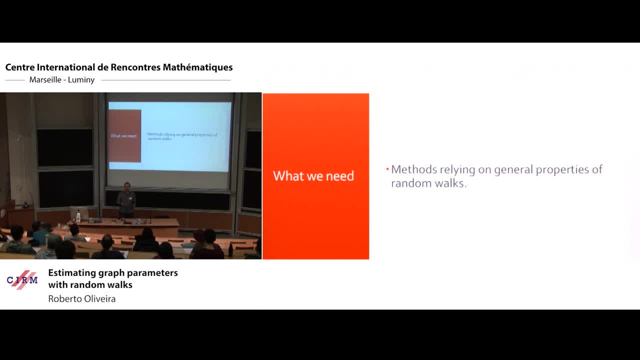 an obvious sentence. We are gonna use random walks, so we don't know exactly which graph we're walking on, so we need kind of general methods. Okay, just to remind you of lazy random walk, I mean, that's just the transition matrix, right? 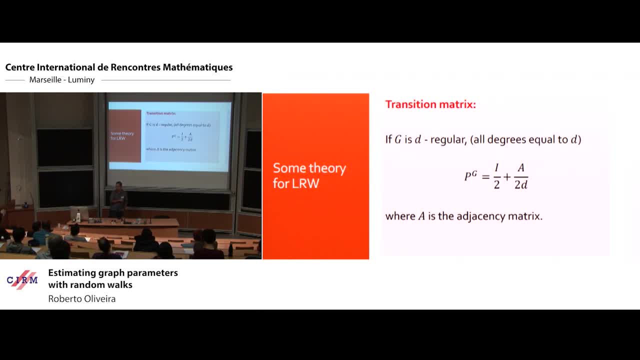 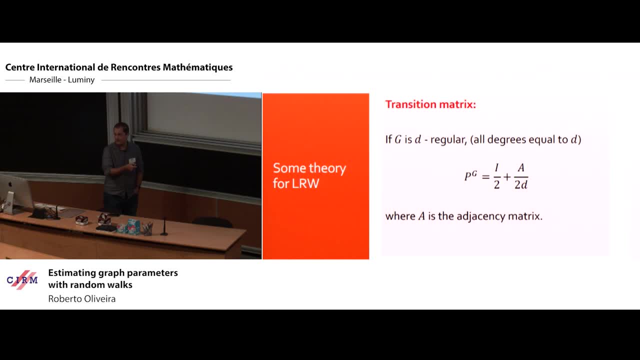 If the graph is regular- and I'm gonna give some proof sketches for the regular case- that's just well. a JCC matrix divided by the degree plus the identity and divide everything by two, right? So this is saying: stay put with probability ahead, right? 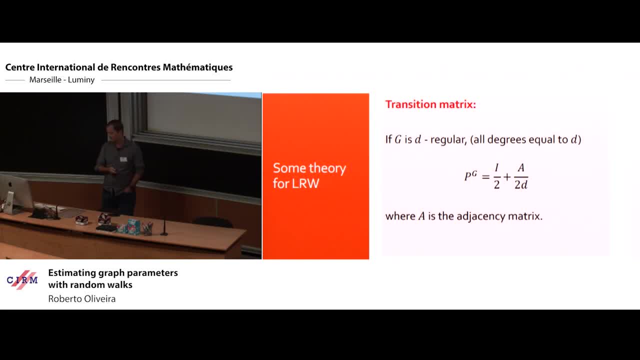 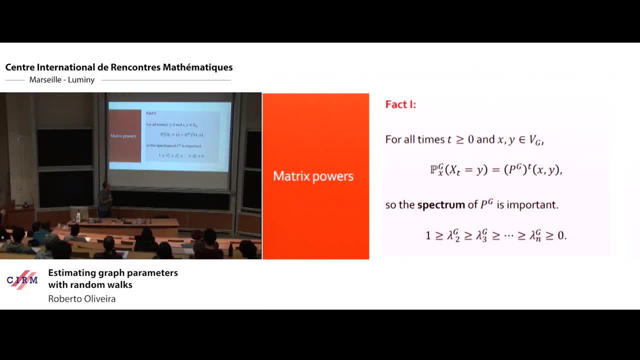 Probability ahead, take a step to a neighbor with probability ahead, And I mean, that's also kind of obvious. so maybe you're almost embarrassed to say this in this audience, right, But we're gonna, because we're gonna be looking. 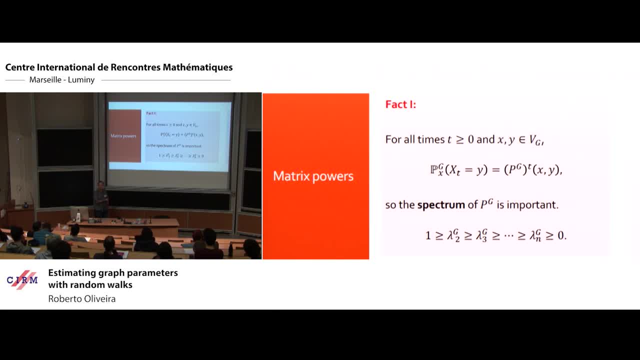 at higher powers of this guy. the spectrum's gonna be useful- and it's nice to know that- for lazy random walk, as I said. I mean the important thing is that the spectrum is no negative. So there are many things that work for lazy random walk. 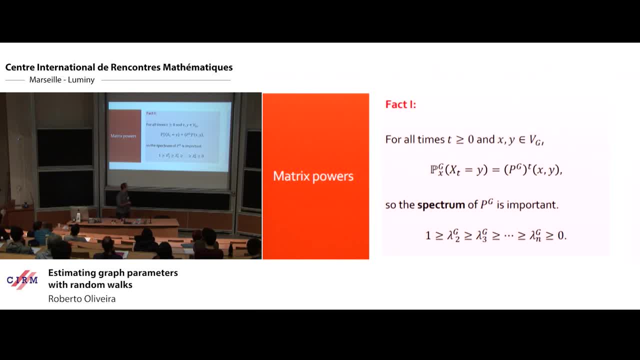 for this reason that don't work. for if you allow negative eigenvalues, right. Well, so you have. I should say you have- a real spectrum, because this P is self-adjoined. well, I mean, if the graph is regular. 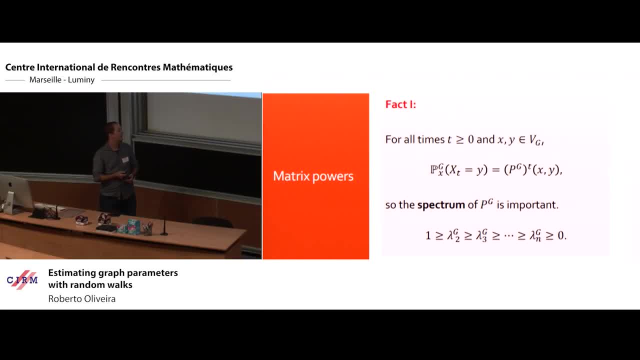 it's really a symmetric matrix, so there's no question about it, And it's a real non-negative spectrum, because random walk's lazy. And this parameter, which is called the relaxation time, is gonna be very important for us. Here I'm only relating it to the Stieger constant. 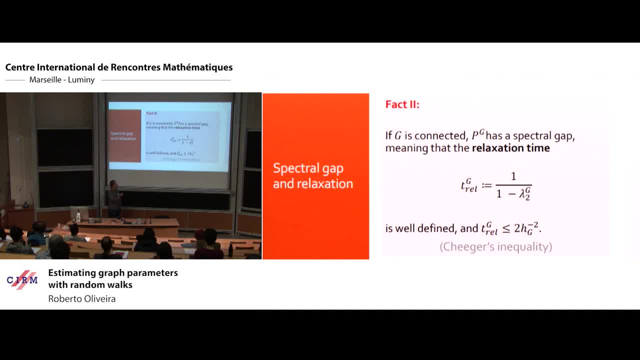 that I introduced before. but I mean, you don't need to think about this, It's just, let's keep this number in mind, And so what we're going to do is basically write upper bounds. I mean positive results in terms of the relaxation time of the graph. 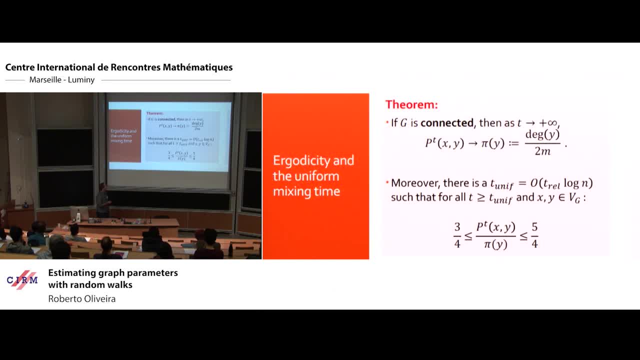 It turns out that's a convenient quantity to look at. Well, there are gonna be a few results that are not gonna be about the relaxation time. They're gonna use the fact that you know, we know that as t go into infinity. 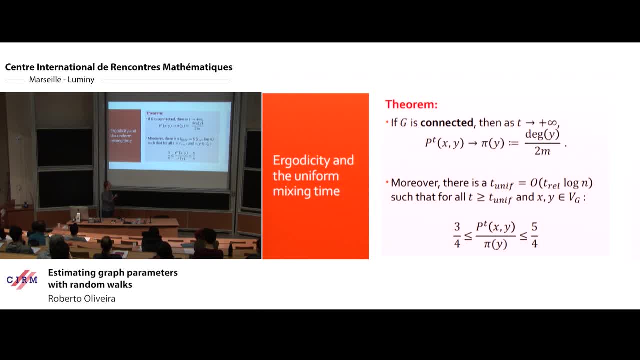 the probability of going from x to y in t steps converges to degree of y divided by twice the number of edges, And we know that there's a time- that's at most the relaxation time times, log n- at which this ratio is close to one. 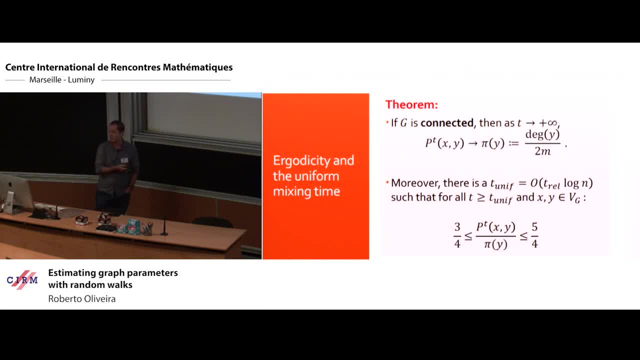 I mean close to one means that it's soft by a factor of at most of a quarter in either direction. So this is what we call the uniform mixing time, But for most things we're gonna be talking about the relaxation time, And maybe I should mention before it continues: 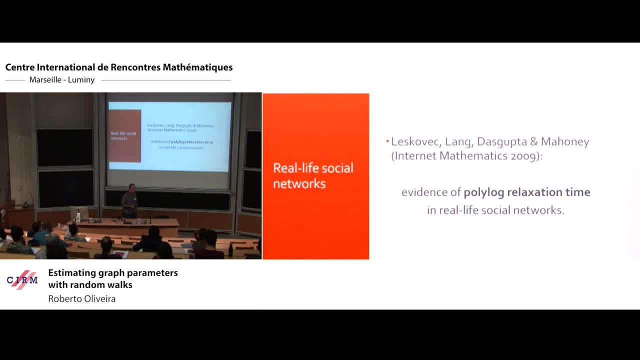 that you know. we're gonna be talking about results that say, well, if the mixing, if the relaxation time is small enough, then you have sublinear algorithms, which are sort of our holy grail, so to speak, And there is some degree of evidence that you know. 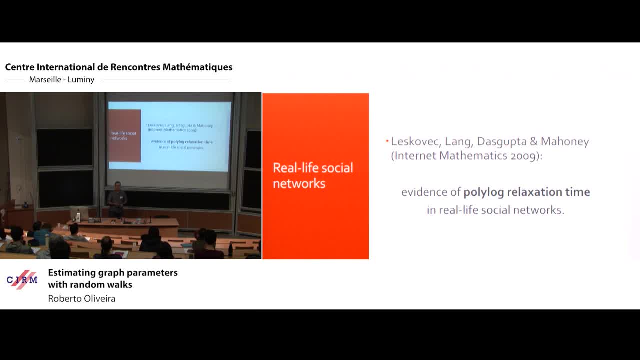 social networks. in real life, they have polylog relaxation times or mixing times, which means that maybe, you know, if I was talking to an audience of you know, an audience of engineers, I could even claim that my results were useful for something. 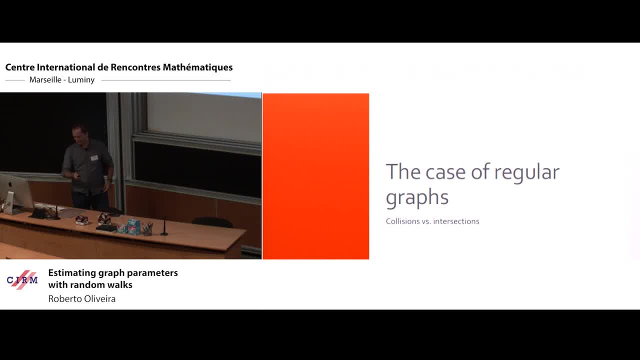 I have nothing against engineers, by the way. Some of my best friends are engineers. Okay, so let me tell you what we do in the case of regular graphs. And then we- and this case is nice because there's- I already mentioned- the birthday paradox- 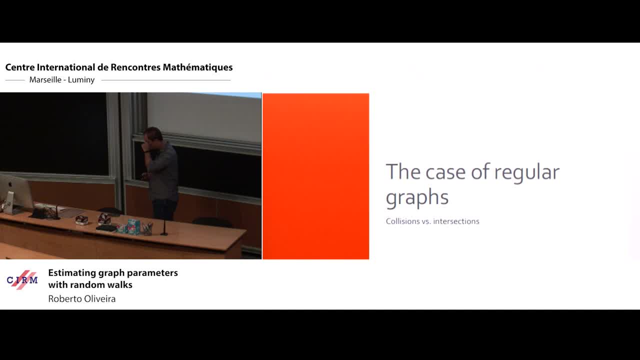 and you see this square root of n bound for expanders, which seems related. So we're gonna see that there's an idea that several groups have tried, which is looking at random walk collisions and trying to use those to figure out the size of the graph. 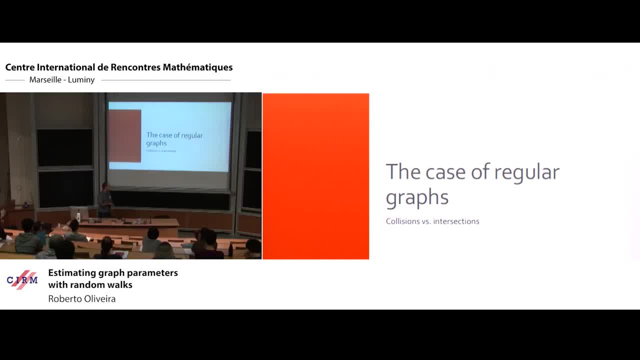 And that's really similar to the birthday paradox, but we're gonna see that what we use, which are random walk intersections, are more efficient somehow. Okay, so we have this: that if you run a random walk for more than 10 univ steps, then if the graph is regular. 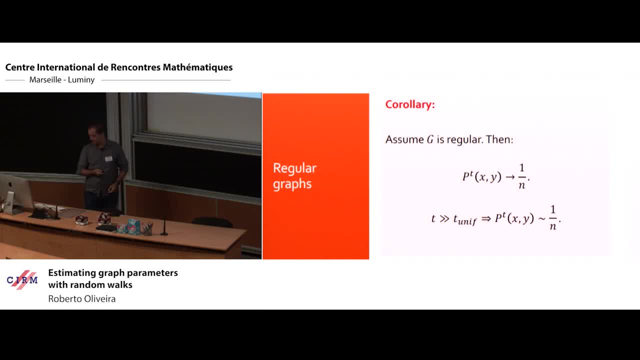 right. the stationary distribution that I showed you is uniform. So if you run a random walk for long enough, you have one uniform sample from the graph. If you run several random walks, loosely speaking, you have an IID sample of uniform vertices of the graph. 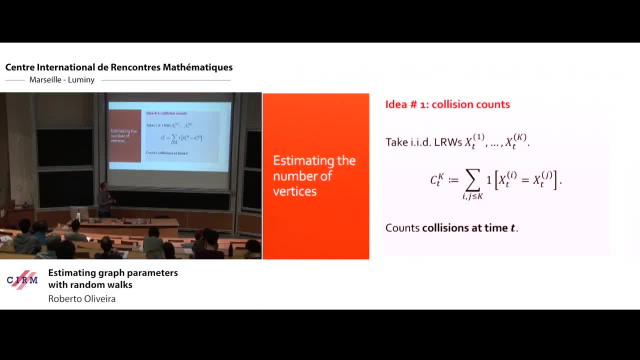 So this is the idea that people have tried, They've looked. I mean, they take their k random walks and they look at how many collisions they see at a time- t, Assuming that t is large enough. you expect that this is like: well k squared. 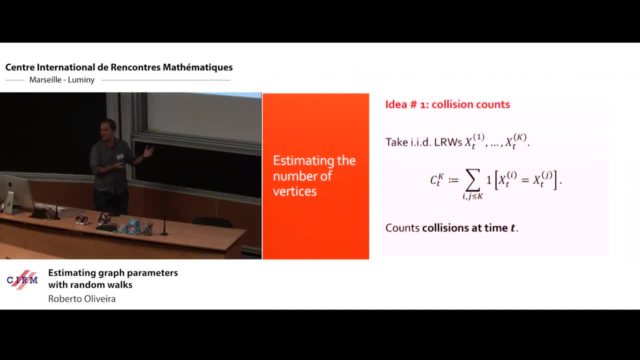 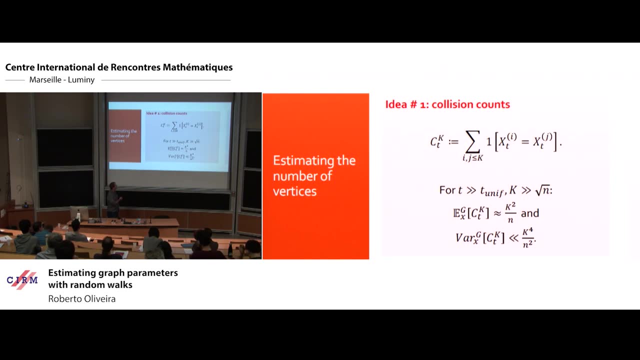 divided by n right An expectation. that's what it, that's its value. So here I should have said that i and j are different, otherwise you get something silly. But yeah, so what happens? is that okay if you take t to be larger than uniform mixing time? 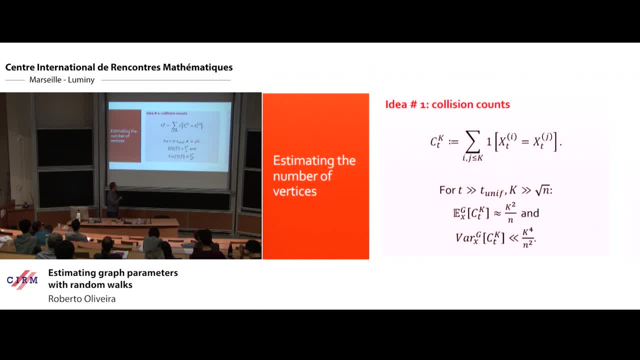 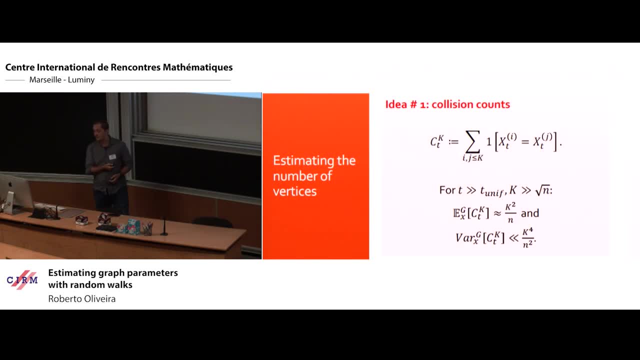 if you take a k that's larger than square root of n, then the expectation of this random variable is k squared over n, and the variance is less than the expectation squared. So what well, I mean? this means that if you do things, 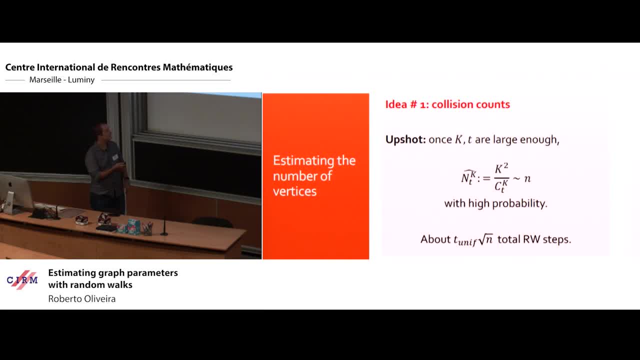 in the right way. you can basically get just by looking at this random variable right. So if k is greater than square root of n and if t is larger than uniform mixing time, if you look at this ratio of k squared to the number of collisions, well, this is typically close. 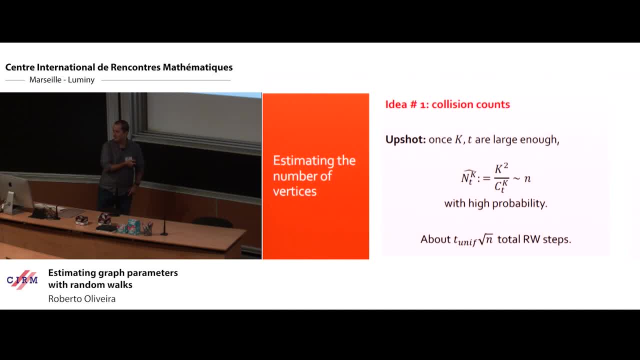 to k squared divided by k squared divided by n, which is n, So great, that's an estimator for the number of vertices And the number of random walk steps that you need. is this right? so you need a number of random walk steps. 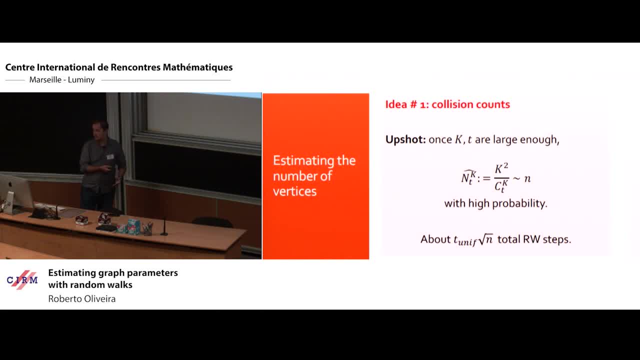 like square root of n at least, and you need a time that's like uniform mixing time at least. But then we can look at our two examples and we see: okay for expanders, that gives you the right result, right. 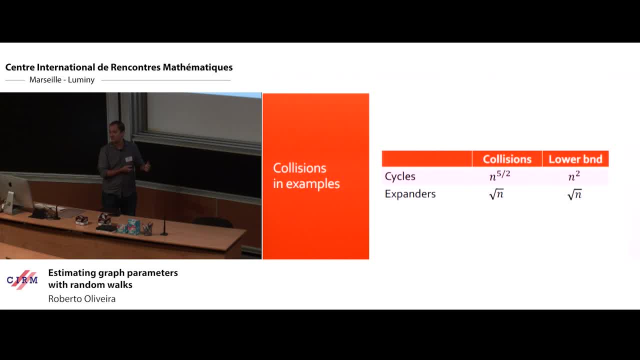 Because the well, almost up to a log factor, right. So we have a lower bound, that's square root of n, and the upper bound, well, the uniform mixing time is log n, square root of the number of vertices, that's here. 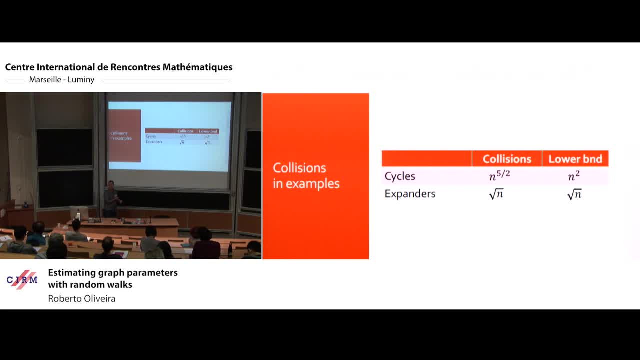 so that roughly matches. But for cycles this is way off. So, but just to mention right. so there are many papers about this idea. there are also papers by Laurent Massuyer and others where they generalize these ideas to non-regular graphs. 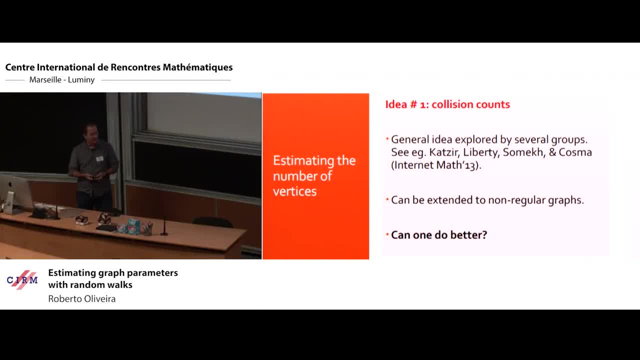 And our main, in some sense our one other motivation that we had is that: well, can you make better use of random walks and try to figure out the size of the graph? If you don't look only at collisions but you look at more information somehow? 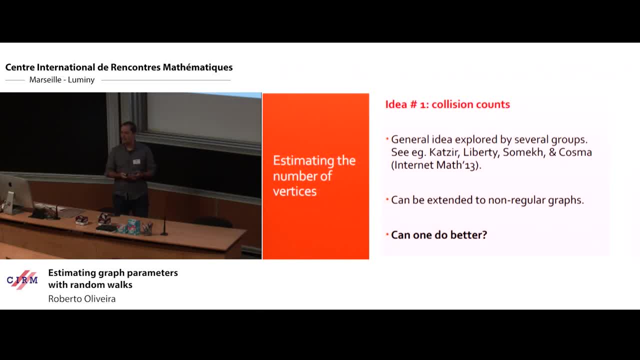 Of course, more information could be anything right, So it's better to have a concrete thing in mind, And we're gonna be looking at intersection counts. So now capital K is twice some small k. We're gonna be looking at pairs of random walks. 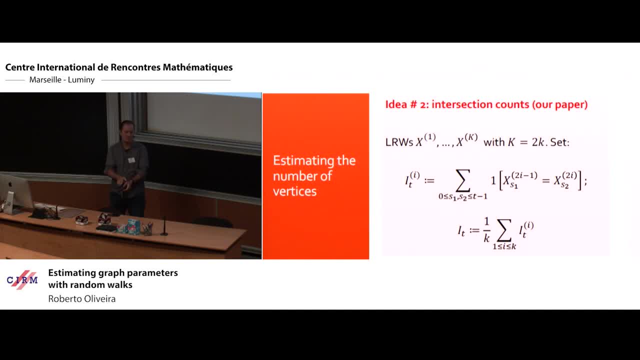 They are independent and maybe I mean we're gonna be thinking they start from the same vertex And and for each pair you're gonna count the number of times the two paths intersect up to time t right And an intersection by definition. 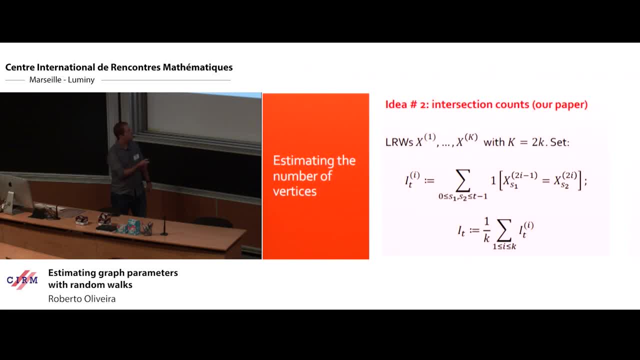 is just a pair of times- s1, s2, where random walk? this random walk is at the same place as this random walk, Right? This random walk at time s1 is at the same place as this random walk at time s2.. 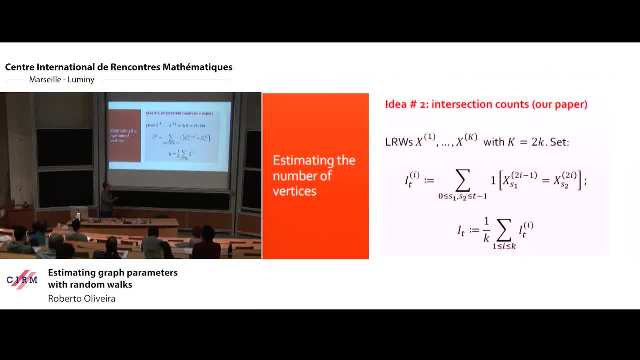 And to get the intersection count, well, we're gonna take an average, just because we're taking a sum of little k values. Okay, what can we say about this random variable? Well, there was a previous paper by Yuval Tomasalva. 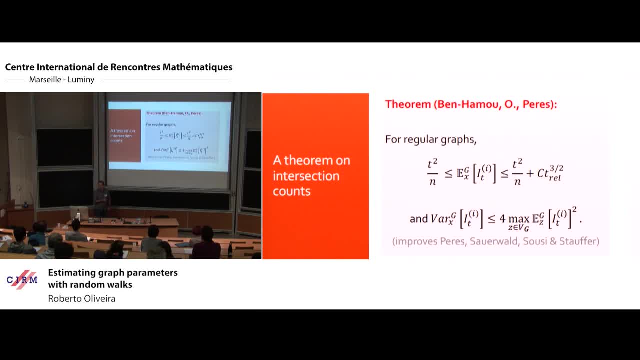 Per Lasusi and Alexandre Stauffer, where they proved some results on this random variable, these random variables in the case of transitive graphs, But it turns out, and it turns out that you can prove this more generally for regular graphs. 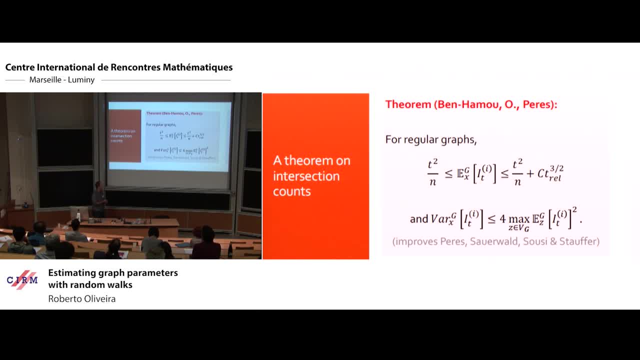 and you can even prove the bounds a little bit in that degree of generality. So what you can prove, okay, assuming everybody starts from the same vertex. so okay, if you count collisions for stationarity right at any time, you have two. 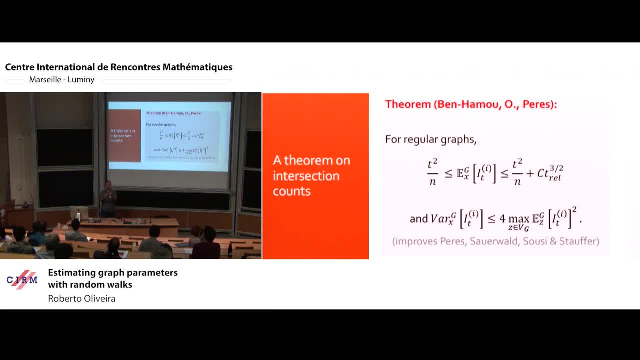 if you have two random walks that are stationary, they probably they intersect at those. not at any time, sorry, at any pair of times. s1, s2, they're probably they're equal with t. sorry is one over n. and because we're counting a number, 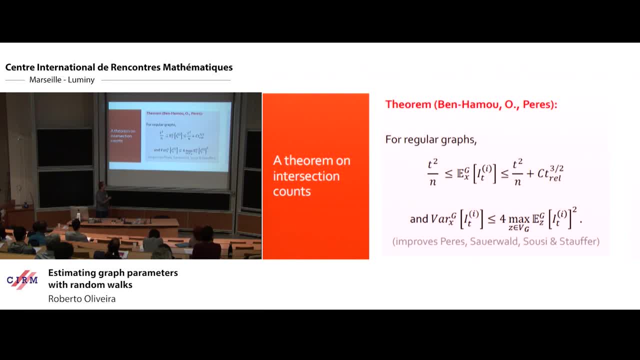 t squared of steps in total, then you have t squared over. n is the expectation when you start from stationarity, And this is always a lower bound for reasons we're going to see if everybody starts from the same vertex, But then you have an upper bound. 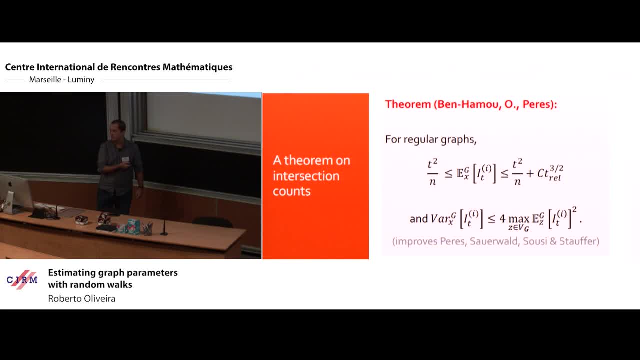 that's the same term, plus this mysterious quantity which I'm going to try to explain, And you see that the variance is at most the expectation, squared up to a constant factor. Well, this is the worst case, but I mean, if you take t large enough so that this is larger than this. 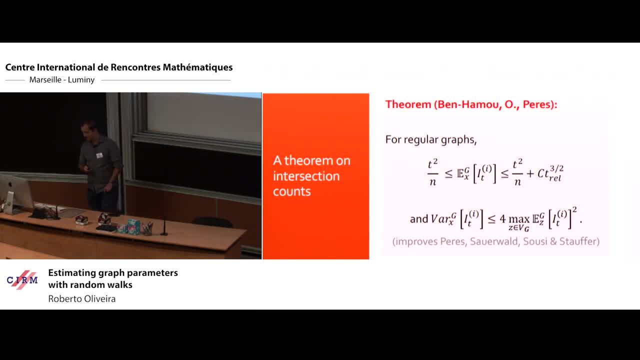 then really everything, sort of matches. Okay, what do you get from this? So, again, as I said, you want to take t to be large enough that this term dominates the other term And that. what does this lead you to? 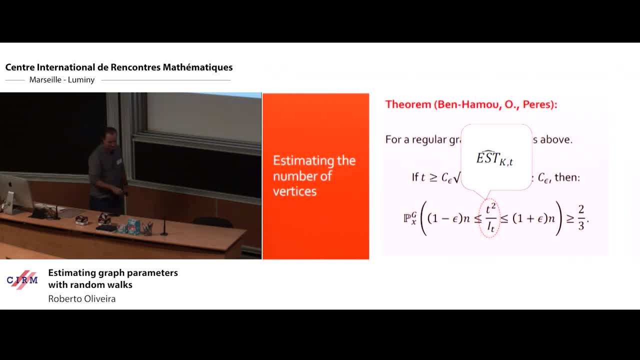 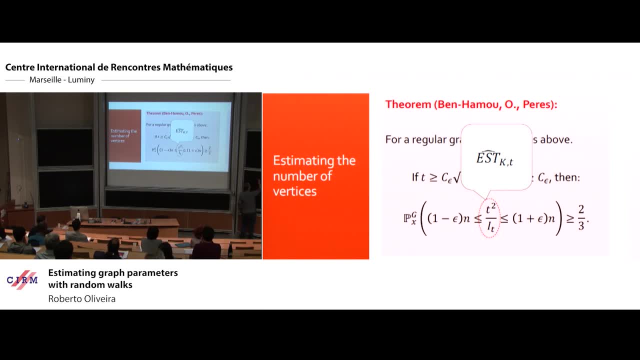 Oh, sorry, that's I'm not sure. yeah, I had a PowerPoint version which wasn't working properly. it had an animation, so let me perhaps write down: I want t squared over n to be greater than constant t rel. 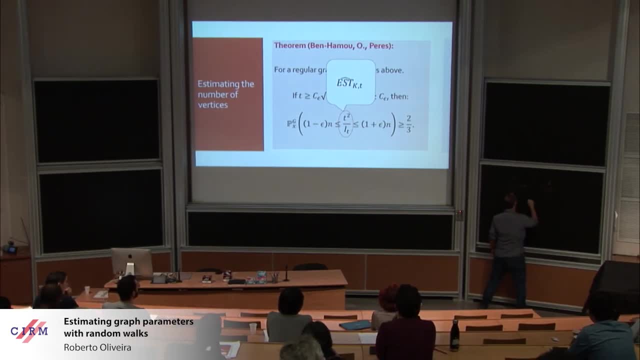 well, let me raise the constants, And so that's the same as saying that I need t to be greater than squared t squared over n, t rel raised to 3 quarters. So the theorem is saying that if I take t to be large enough, 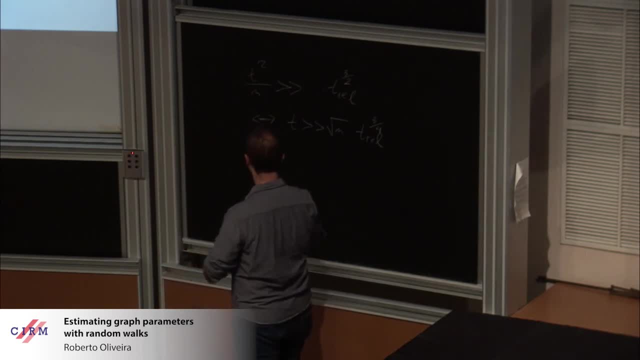 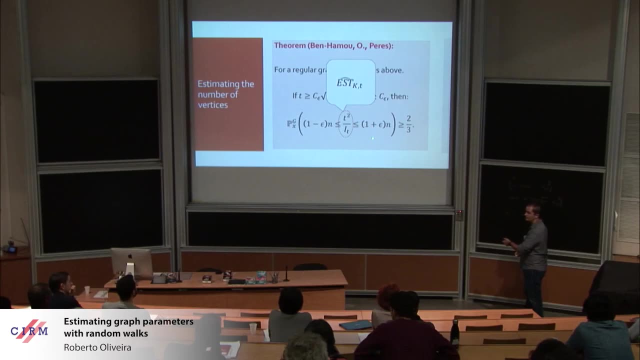 and I also need to choose k, the number of random walks. right, so the number of random walks is only going to depend on this parameter epsilon that I have here for the bounds. If I take these two things, then I can say that. 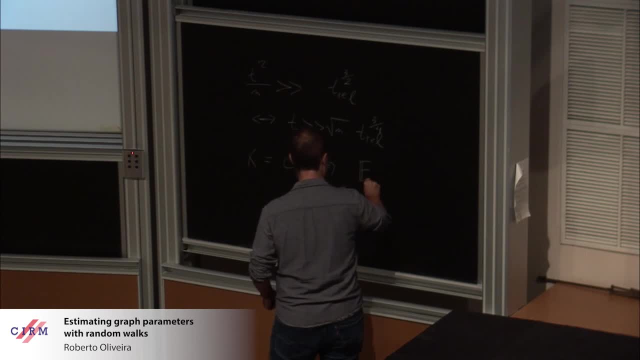 well, okay that I have the expectation of intersections is one plus or minus epsilon, t squared over n, and that the variance- remember that this i sub t- is an average right And the variance is gonna be like the expectation squared divided by k. 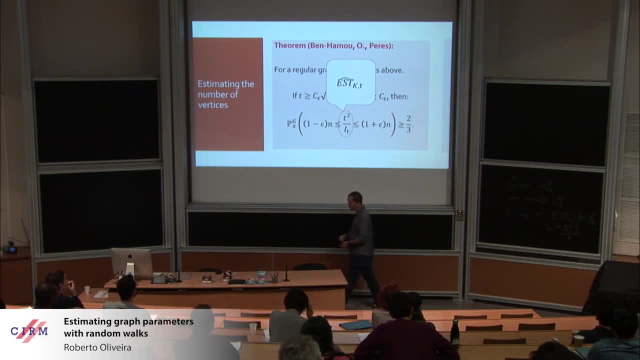 And then, if I do things right, I can prove with that we're probably greater than 2 thirds. the ratio of t squared to this random variable is gonna be close to n, And so that's our first kind of real result in some sense. 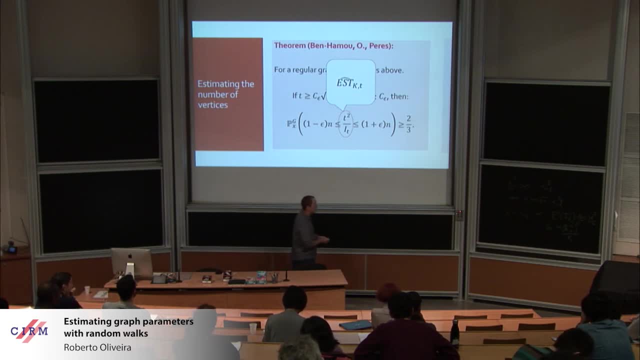 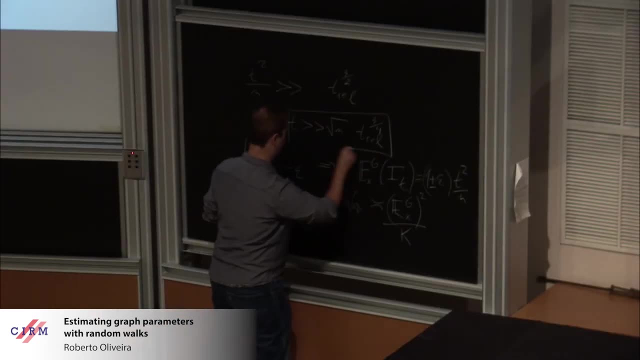 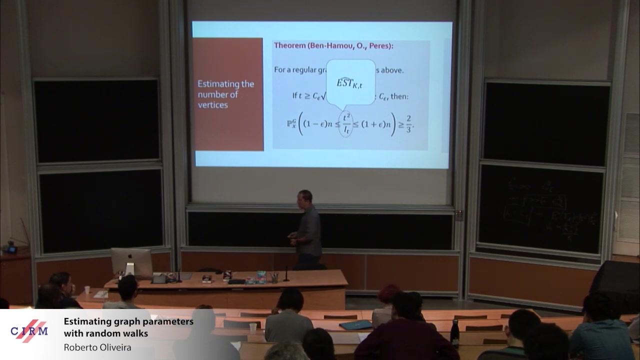 So that's saying that this: if you look at the total complexity- right, so think of epsilon as a small constant- then the total complexity is dictated by these two guys and really the constant doesn't matter. so you get this. In particular, if the relaxation time is less than 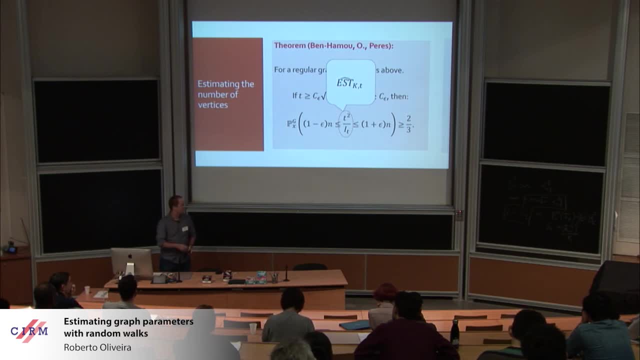 some power of n, which is what is it? I don't know. anyway, If it's less than some power of n, you get sub-linear. And let's compare this idea to the collisions idea, which so it's saying that you have. 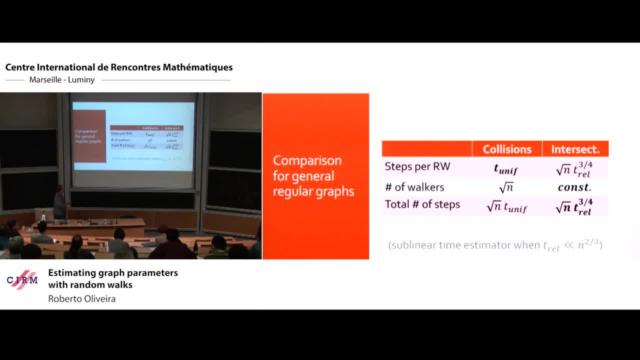 okay. for collisions you need. the number of steps per random walk is the uniform mixing time. So you have a number of steps. that's usually larger for intersections, right? Each random walk walks for longer The number of walkers. for collisions: the number of collisions is larger. 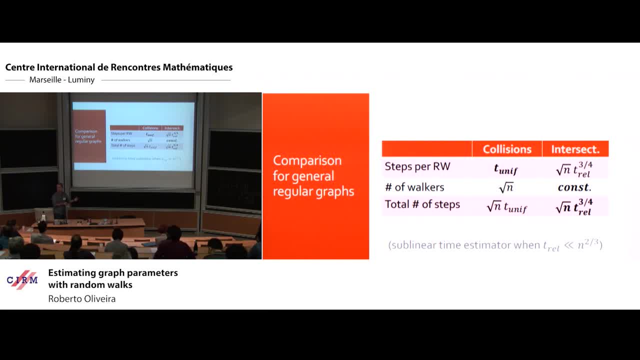 but the number for intersections is a constant for any fixed epsilon. What's the total number of steps? Well, here you get square root of n tunif. here you get square root of n? tral to the 3 quarters, which is better right? 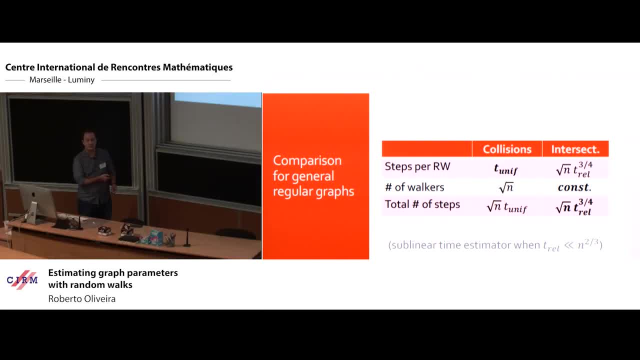 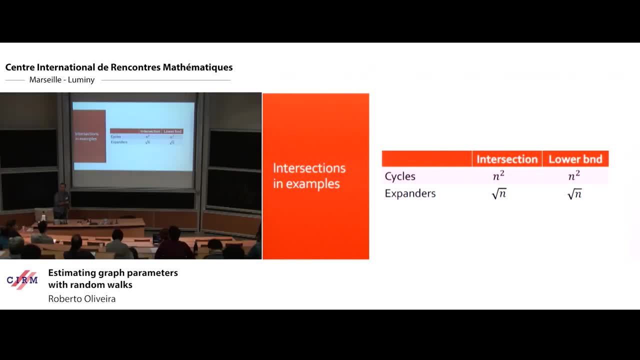 because tral is a lower bound for tunif, essentially. so this is better. And if we look at the two examples we had, so it turns out the intersections give you the right or the order of magnitude, So it just well for cycles. 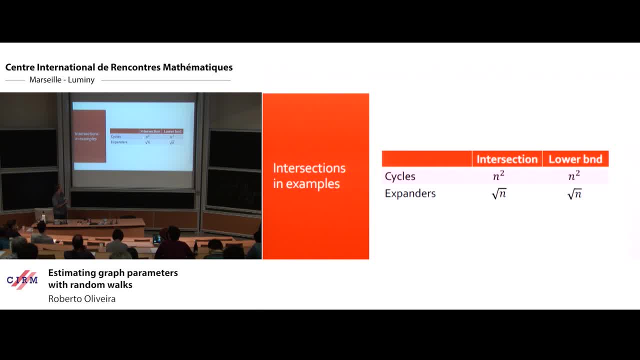 the relaxation time's n squared and you plug it in there, you get n squared For expanders. you know collisions are already good. this is also good. But a more interesting question, I mean, since we write bounds in terms of relaxation time. 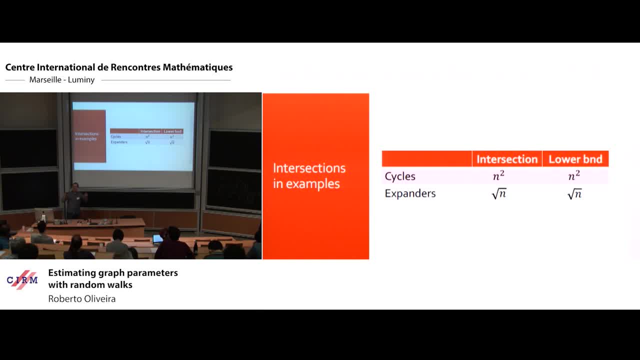 we should say have a lower bound. that says something to the effect of for any value of relaxation time or for any growing function of n, if your relaxation time's at most that function right. so if that's the family of graphs that you have, 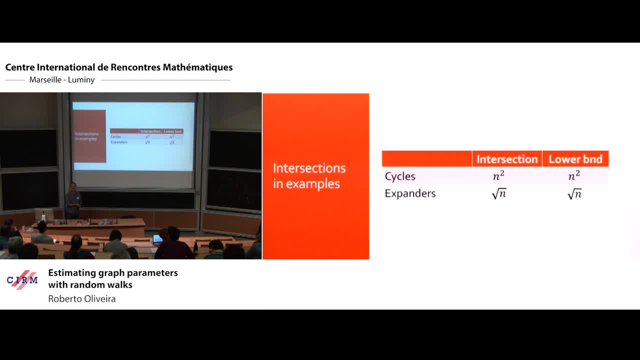 can you prove a lower bound that matches this? So I don't want things just for cycles or expanders. I want things that are in between in terms of the relaxation time. And here's how you build these lower bounds. So I take an expander, that's the. 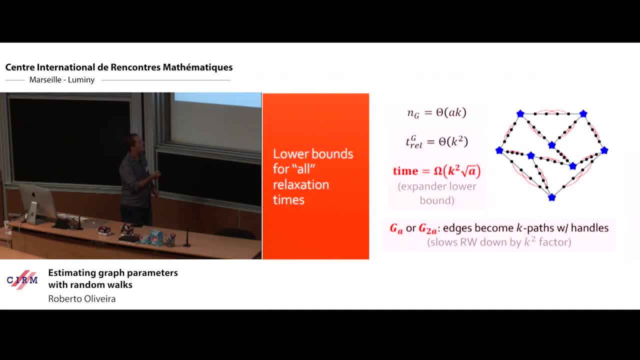 those are the stars here. but the expander has a or two a vertices right. So we know that if we only had the expander, it would take us time, square root of a to distinguish between the two right. that's the lower bound that I showed you. 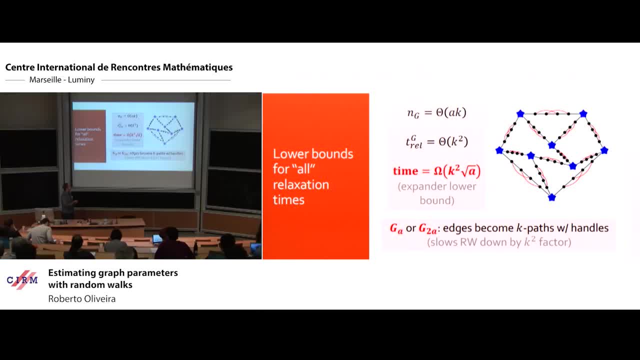 That's the lower bound that I showed before, But now you wanna get a larger graph. so what you do- basically what you're doing here- is you're subdividing each vertex, each edge- sorry- into a path of a certain length: k. 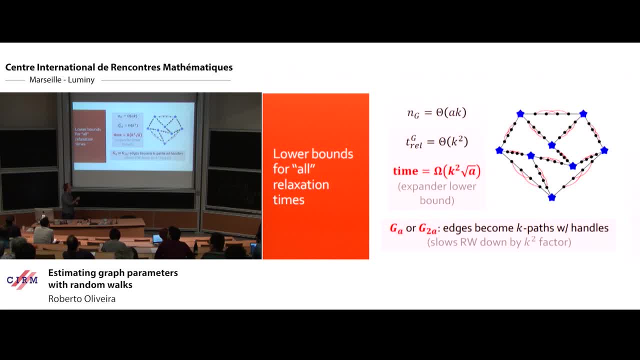 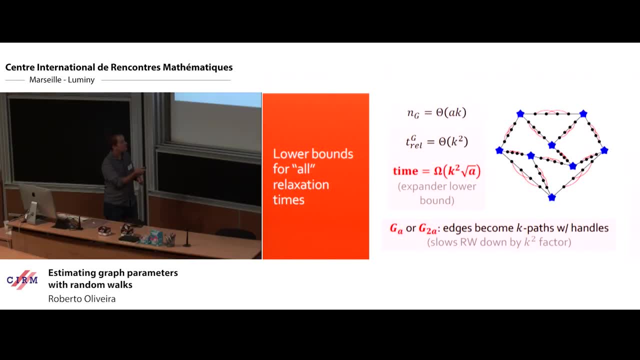 but you wanna keep the graph three regular, so you add a few edges like: well, you take a k, that's okay. so it's really turning. you're adding k vertices on each edge of the original graph and then you connect guys at distance two. 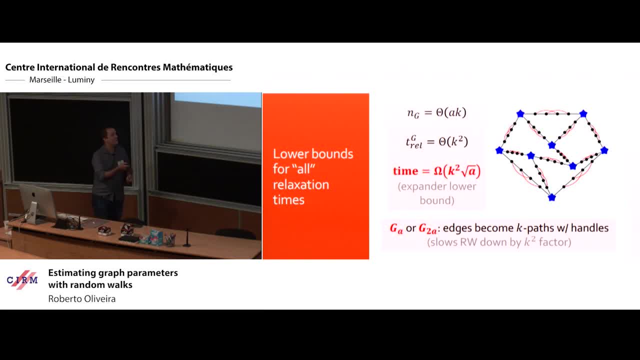 so that you still have the three regular graph. So maybe you need k to be a multiple of four for this to work, but that's not a big issue, Okay. and then you ask: okay, what's the number of vertices? Well, that's clear, right, because you have a vertices. 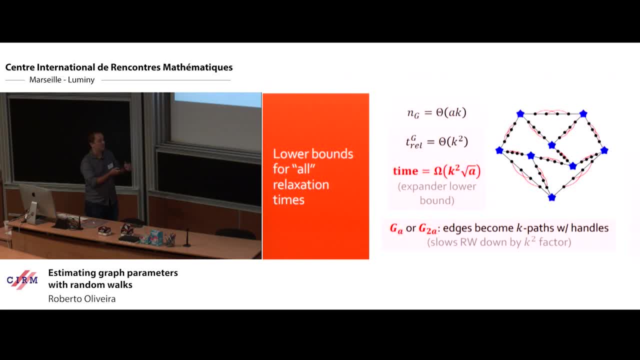 a edges and of the order of a edges anyway. and then basically what you get is a times k and I mean, if you look at it carefully, you get, you know, different numbers depending on whether you have a or two a. 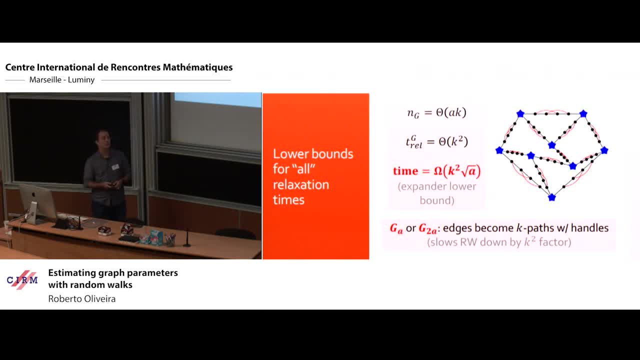 but that's the order of magnitude. What's the relaxation time? Well, we know that random walk takes, on average, k squared steps to cross such a path right. So, basically, random walk on this new graph is random walk on the expander, slowed down. 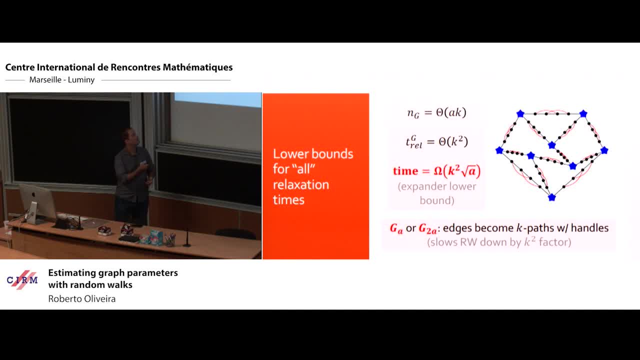 by a factor of k squared and you fork out the details and you can get a bound for relaxation time that's like k squared, and then you can ask yourself what's the time? I need to distinguish between these two graphs, right? 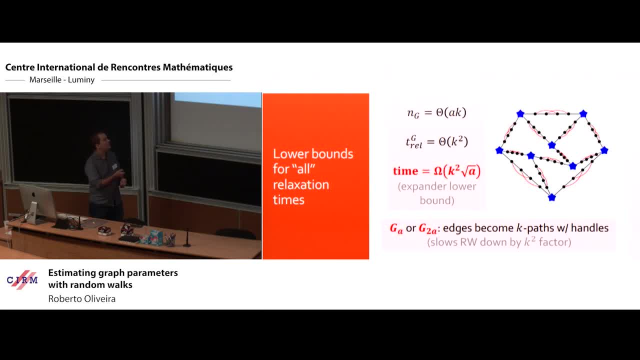 So for expander was squared of number of vertices. Here it's really like random walk on the expander, slowed down by the fact that it takes you k squared steps on average to move from one vertex of the expander to another and you can show. 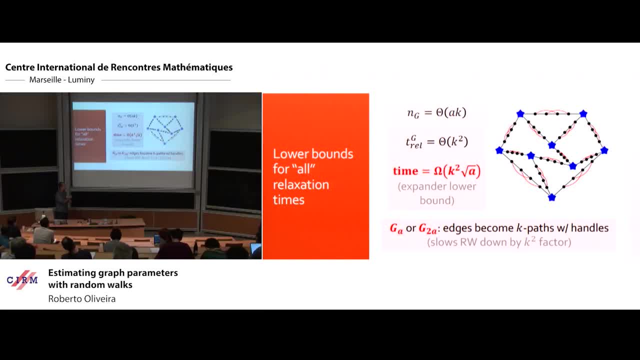 that. then you take at least k squared times square root of a steps to figure out the size of the graph, and then you can look at this: Well, this exactly matches right. you can put a k inside so you get k to the 3 1⁄2 square root of number of vertices. 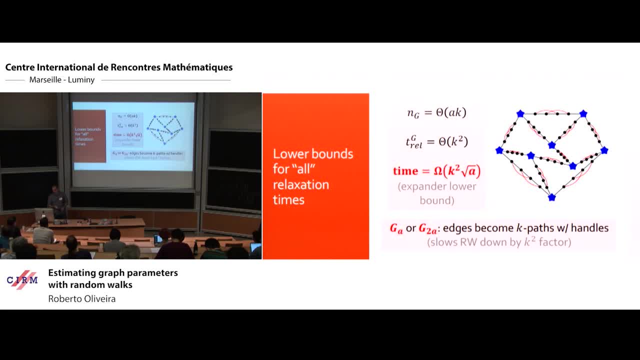 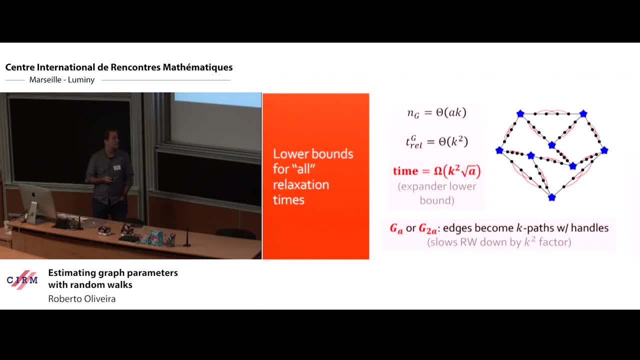 k to the 3 1⁄2 is really relaxation times. k squared right, So you get relaxation time raised to 3 1⁄4.. So it's nice, and in a sense surprising, that this exactly nails the complexity up to constants. 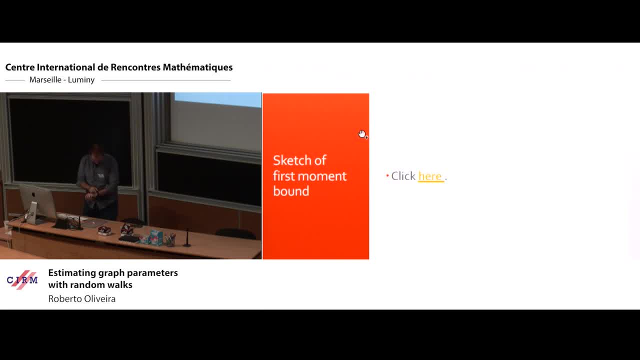 Maybe I'm gonna- yeah, I'm gonna- spend a little bit of time. let's see how much time I have. I'm gonna spend a little bit of time showing you how you prove this and then, in the non-regular case, 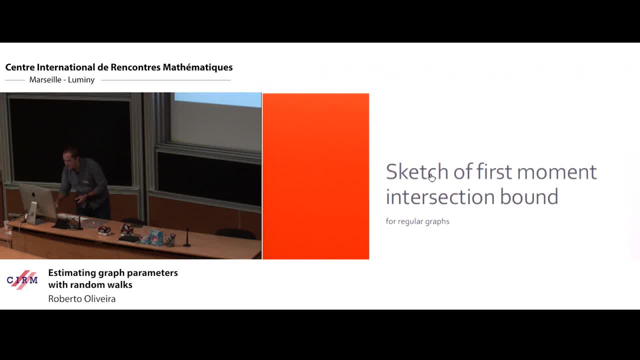 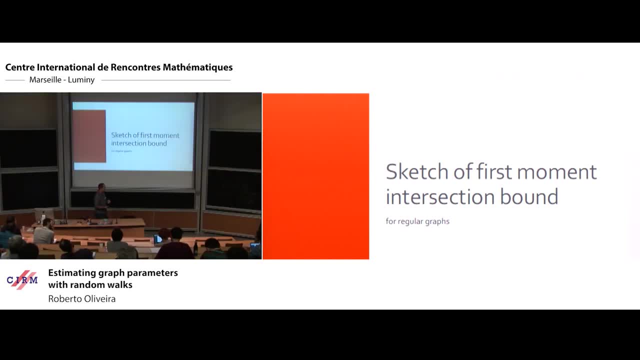 I'm not gonna give proofs, I'm just gonna give you ideas. I mean basically how you build the lower bounds. So what I'm gonna do is really to you know, I've already bragged about the fact that my talk is the most on-topic one in the entire conference. 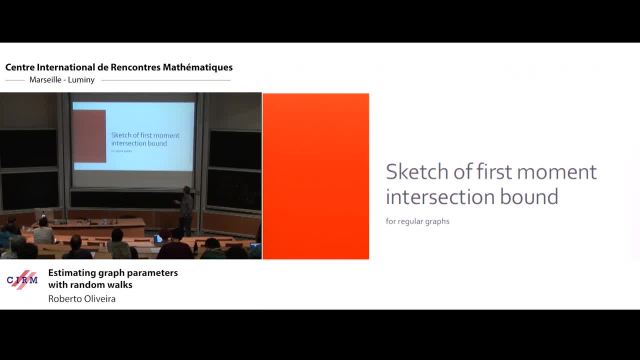 and now I need to show you why, right, Right. so I'm just gonna show you. I mean, I claim these upper and lower bounds for the expectation of the number of intersections between two independent random walks started from the same vertex, x, right. 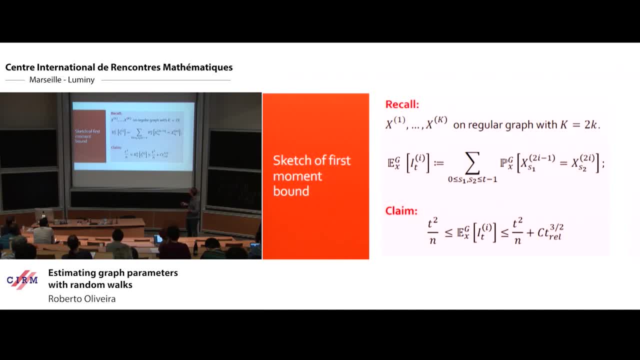 How do I compute this expectation? and then how do I find the bounds right? Well, computing the expectation in terms of the transition matrix is really an exercise, right, It's an exercise in elementary Markov chain theory, And here it is right. I want the two random walks to meet. 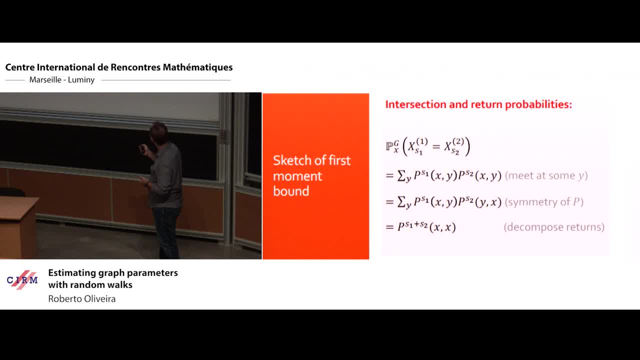 well, I mean at this one at time s2 to be at the same place as the one at time s2, so I just divide into the case. well, they both happen to be at y. Now I'm in the regular case, right? so the 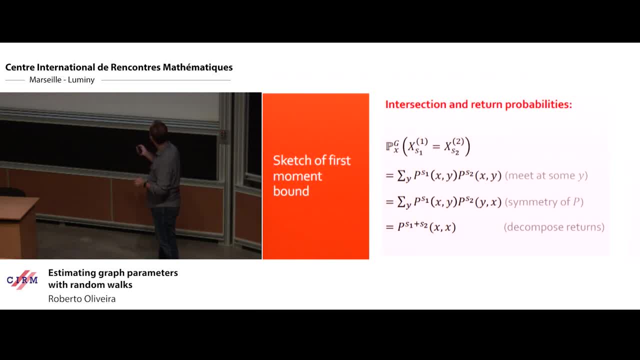 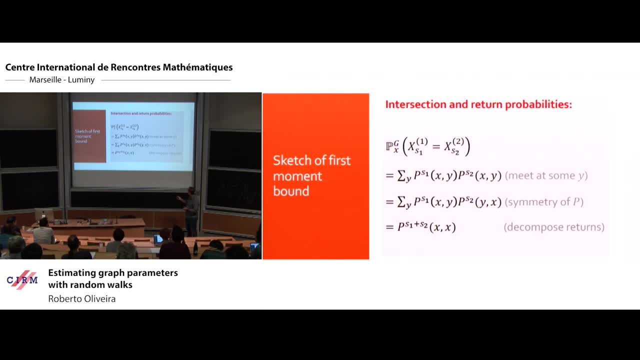 basically p is i plus the adjacent matrix, so it's symmetric. so I can flip and if I look at this, it's just a probability that I go from x back to that. I return to x in s1 plus s2 time steps. 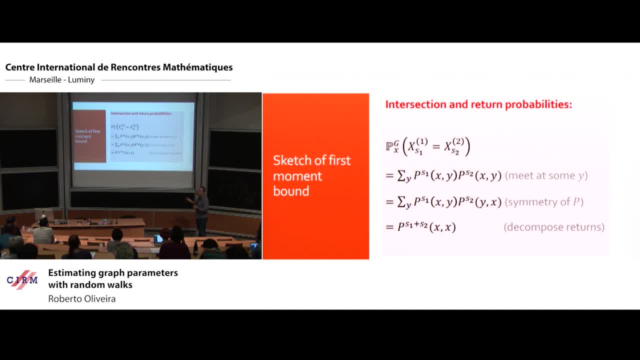 Right, I'm just kind of writing this, probably in terms of where I am at time: s1.. Okay, so this is a bound, but this is well, this definite. but we also know, because we have this non-negative spectrum, that I can write this in terms of eigenvectors. 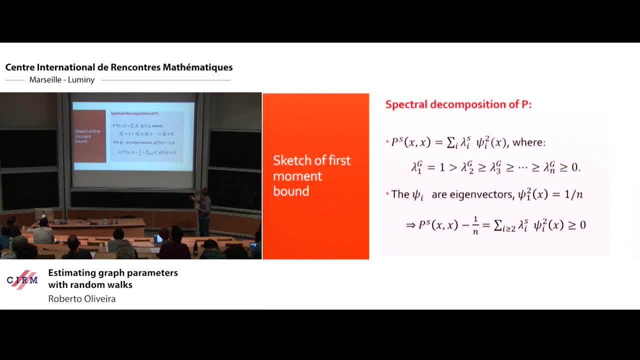 and eigenvalues, right, So this is just linear algebra. I mean, you just have your eigenvectors. you know that the first eigenvalue is one by first, I mean the largest, and that the first eigenvector, when you square it, you have one over n. 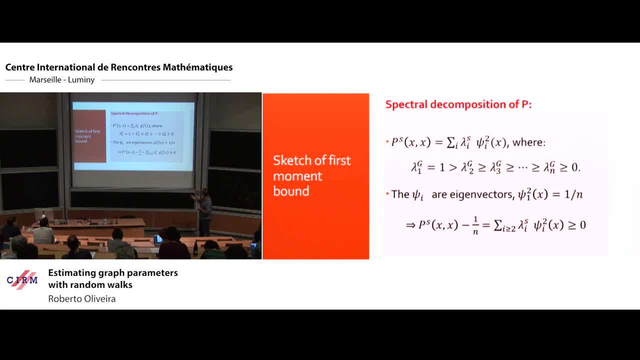 So the first term in the sum is one over n, and then I have a bunch of other terms. I mean, the important thing for me is that the lambda i's are all non-negative and the psi i's well, they're squared. 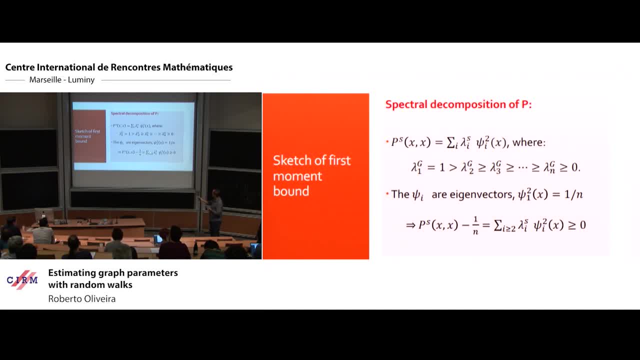 so they're also non-negative, right. And then I look at this and I get this quantity right. I'm summing now, for i greater than two and this is certainly non-negative. So this is why you have a lower bound for the expected number of intersections. 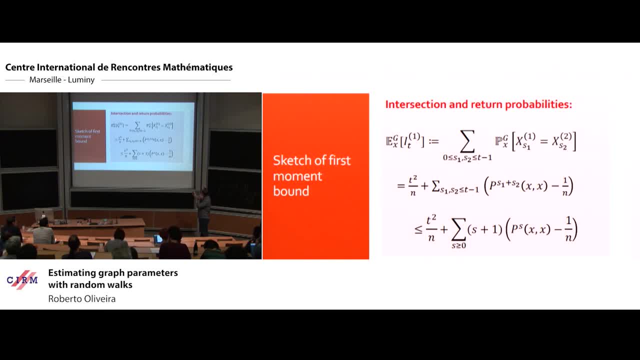 Okay, so far, so good. I haven't done really anything special, so let me just say: okay, this is a probability of return. Then I subtract this one over n factor and I get this t squared over n. As we said, this is non-negative right. 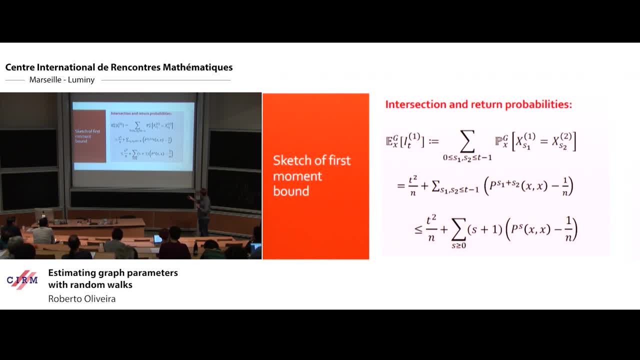 So this is where the lower bound comes from, And also because it's non-negative, I can just take an upper bound here and I'm just gonna say: well, instead of summing over s one and s two up to t minus one, 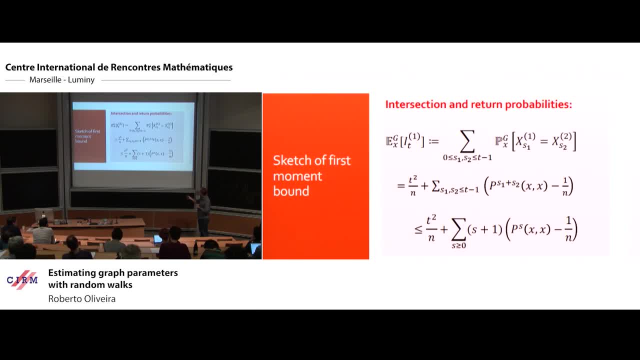 I'm just gonna say, for each value of s, I have at most s plus one choices here That give me s one plus s two, equal to s, and I take an upper bound. Again, I'm using the fact that there's no negative right. 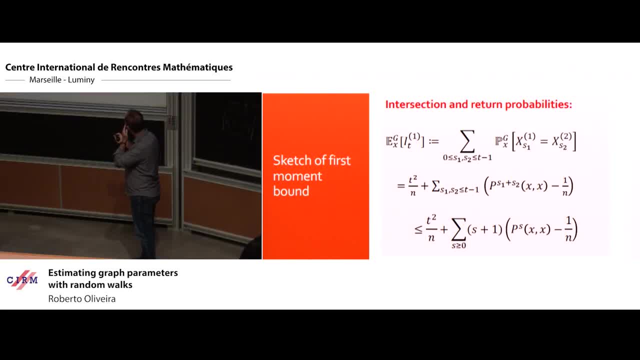 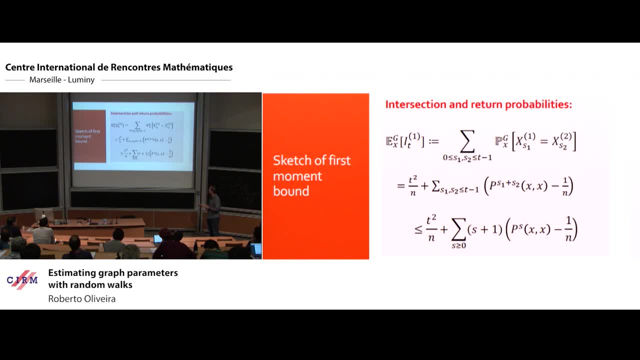 Okay, so what do we do with this? So now you need a way to estimate this and, if you remember, this should be something like the relaxation time to the three halves, for whatever reason. So what we're gonna do is just look at the sum. 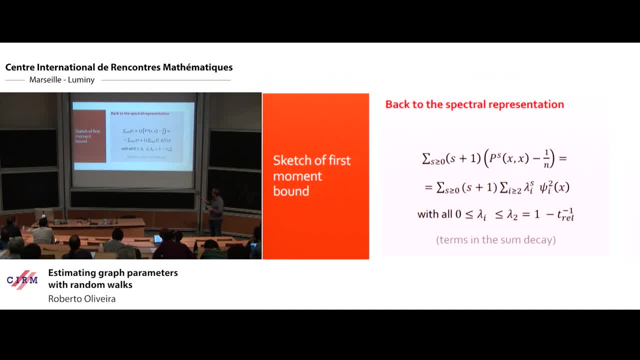 So what we're gonna do is just look at the sum and you have this. I'm gonna write this again in terms of the spectrum and the eigenvalues, And the important thing is that all these coefficients, well, they're less than lambda two. 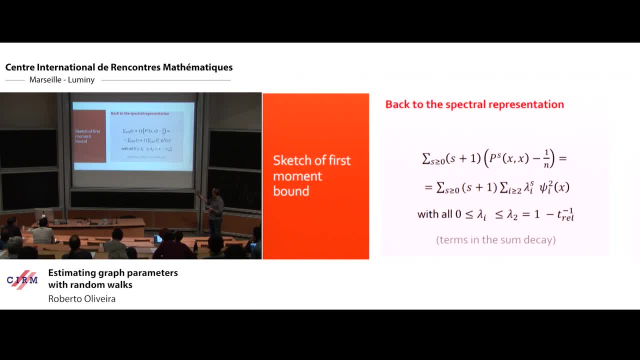 because I'm summing from: i greater than two When lambda two is this guy here? one minus the reciprocal of the relaxation time. What I'm gonna say about the sum, I really don't wanna do anything too fancy. I'm gonna say that if I truncate the sum, 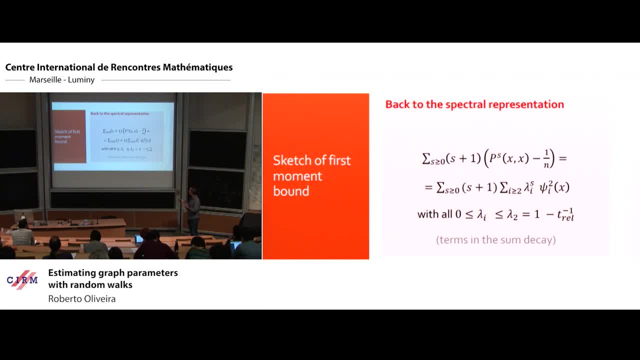 at the relaxation time, then I only lose a constant factor And basically this comes from this geometric decay, right? So it's saying that if I sum, say from, i equals zero. sorry, if I sum from s equals zero up to the relaxation time. 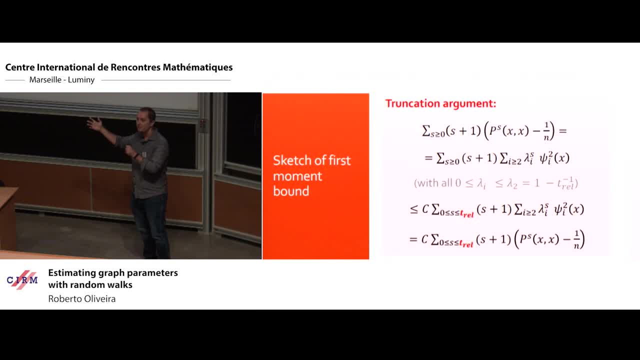 and then I sum from the relaxation time plus one up to twice the relaxation time, say the second sum is at most a certain c times the first sum and the c is less than one. That's basically it. I'm saying that you know. 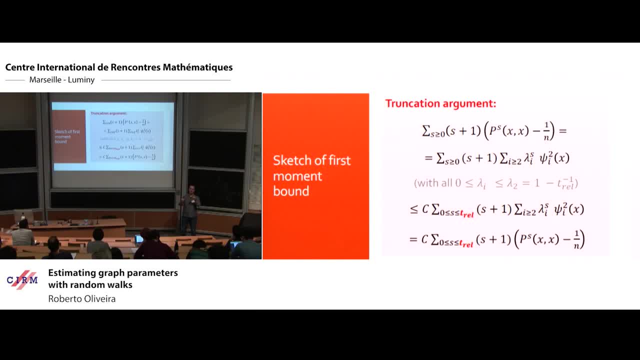 I divide my sum by one, I sum into chunks of size the relaxation time, and each one is geometrically smaller than the previous one. So, and then I get up to a constant, so I get. I can just sum up to relaxation time. 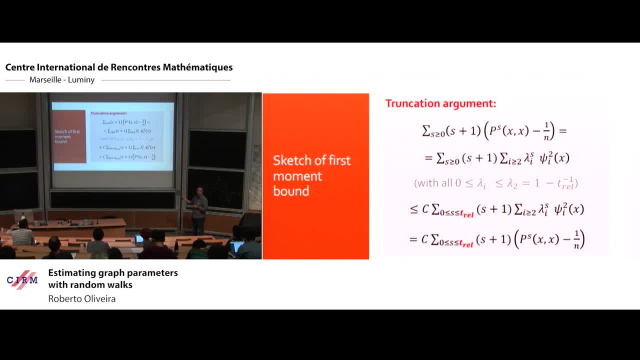 And now there's this one last step, which is: how do I estimate this guy? Now you can go back to this to say, Aldous and Phil, this book that's been in preparation for forever And there's this bound that tells you: 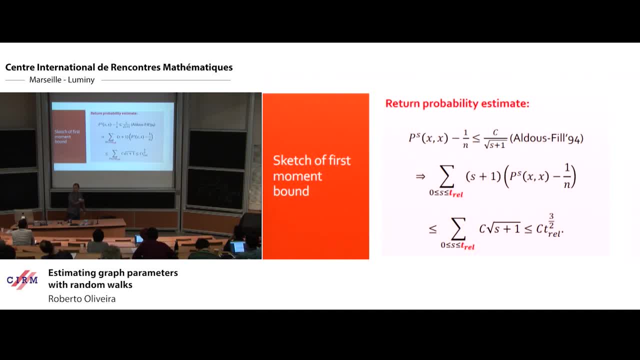 that this difference is that decays at most like one over square root of s, And if you plug that in, you get here well, s divided by square root of s, so you get square root of s, and this is where you get the T? rel to the three halves. 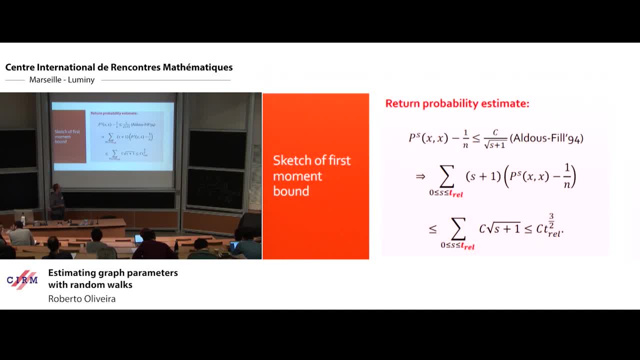 Okay, that's. I probably showed you too much, but that's just to give an idea that first we need some general tool to truncate this expansion and then we need something very specific. I mean, this is, of course, sharp for paths, right. 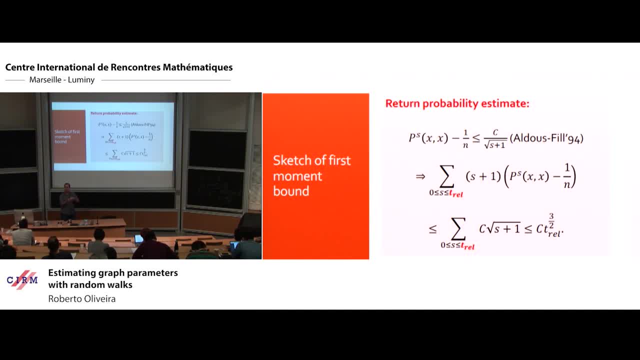 So, in a sense, it's not surprising that our lower bounds come from graphs that have long paths in them. right And yeah. so just to say I mean, if you wanna do it, yeah, so that's the end And right, we just bounded this thing. 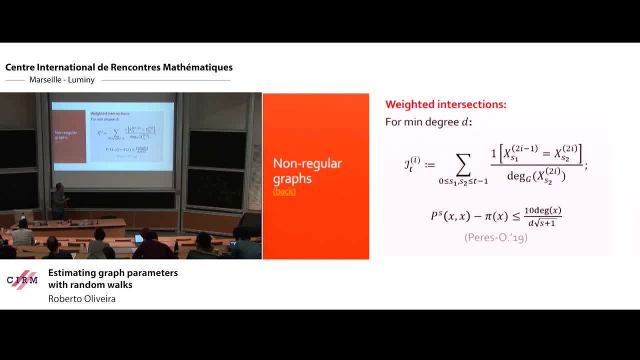 And now I mean, if you're gonna do the non-regular case, which I'm gonna be talking about in a second, we're gonna be looking at slightly different bounds for this that work for non-regular graphs. So this is the degree of the vertex x. 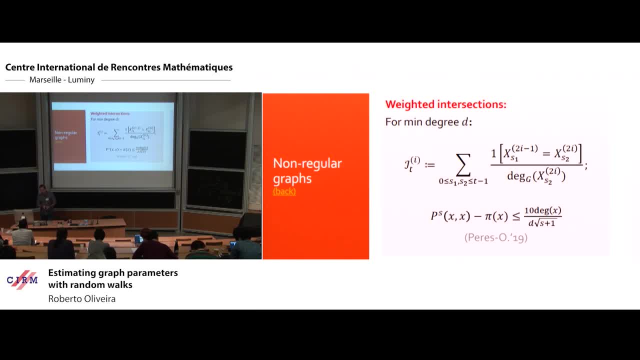 divided by the minimum degree in the graph. And these bounds are new. I mean, we proved them in a separate paper, Right? let me just go back to the core of the talk. So I hope I have convinced you that this result. 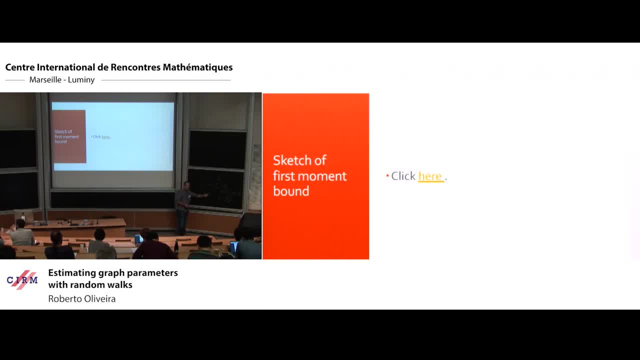 I mean the upper bound. at least the expectation here makes sense, right, And, as I said, it has everything to do with the spectrum, though we don't use much about the spectrum, we just use it, that's no negative. 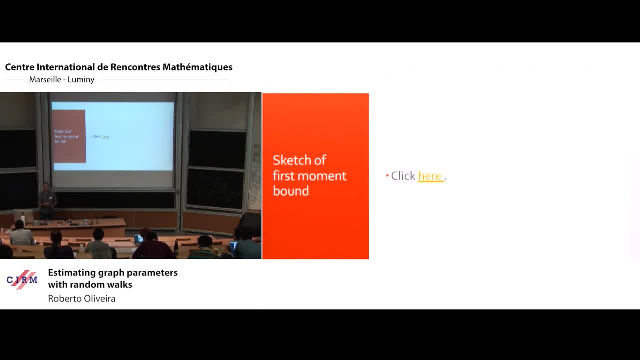 and that all eigenvalues, except the upper bound, except the trivial one, are dominated by one minus one over T rel. And then, okay, we need this one last thing, which is this decay of the return probability. Okay, what's the message of this part of the talk, anyway? 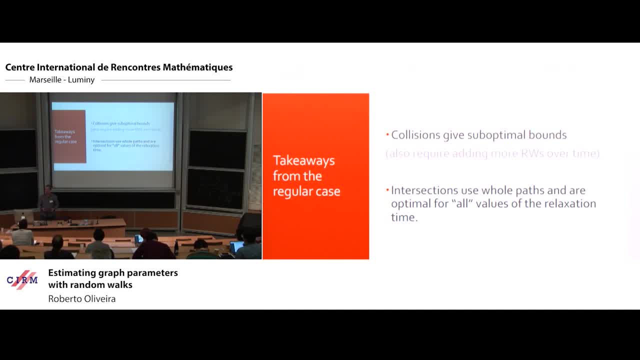 Is that collisions are a very natural idea because we understand them very well, but they turn out to give you suboptimal bounds And these intersections give you well- I mean they use more information about the Rhen walks right. 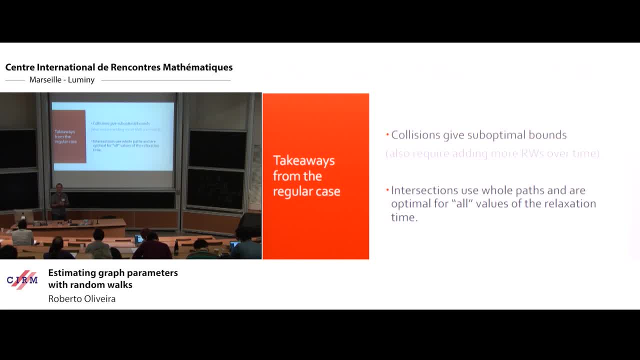 They don't look at what happens at time T, they look at what happens at all times up to T and it turns out that they're good enough to give optimal bounds for all values of the relaxation time. Right, but of course we want results. 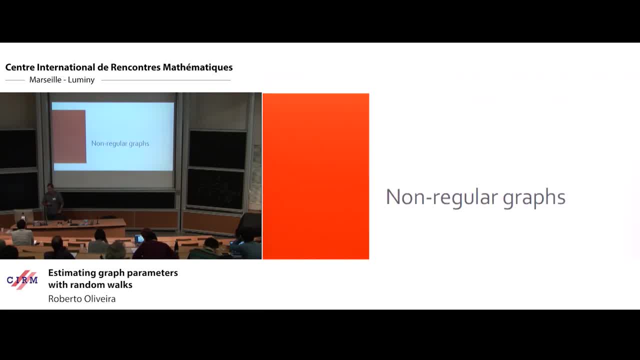 for non-regular graphs, so I'm gonna go quickly through them. Okay, so you've seen this proof, or this proof sketch for the bound for regular graphs of number of intersections. right, If you try to make that work. 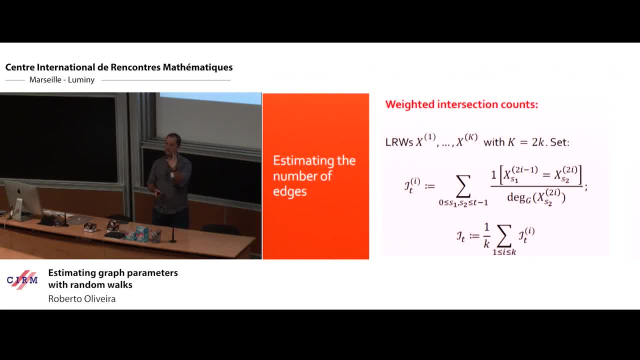 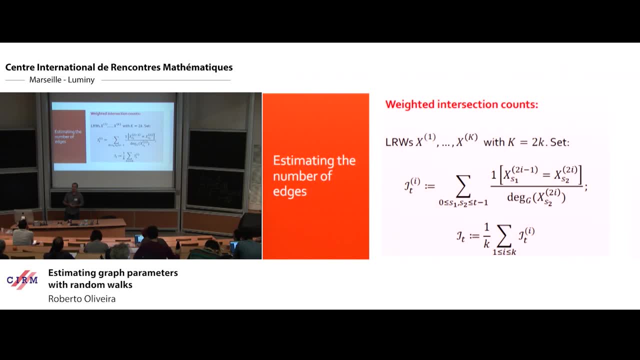 there is a crucial step in the proof, which is symmetry right. You need to flip the JSC matrix. Symmetry doesn't hold for general graphs, but something called reversibility, which probably all of you know holds. And if you wanna make that work, 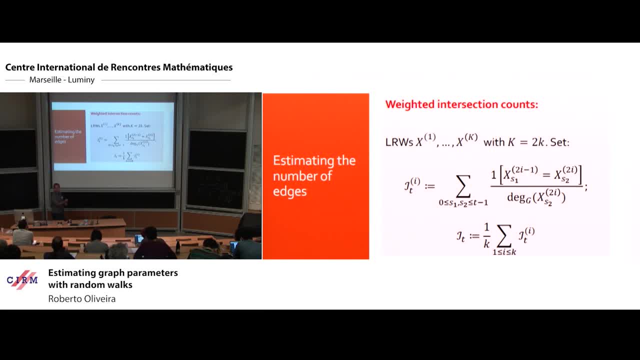 it turns out that the crucial thing is to weight the number of intersections by the degree. And the question is: I mean this is not gonna give you the same boundaries before. What does it give a bound for? Well, following the same proof, 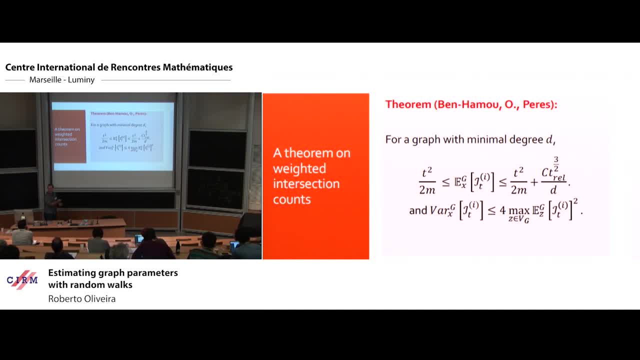 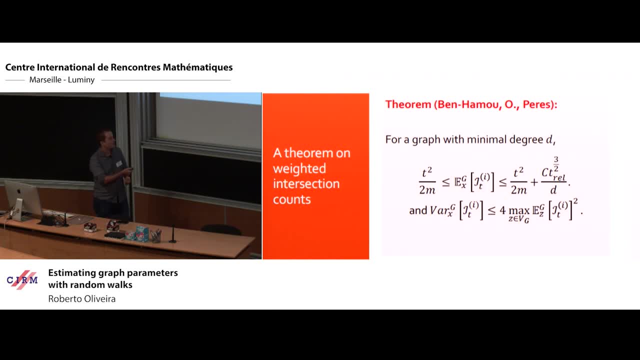 you see that instead of getting n, the number of vertices in the denominator, you get two m, twice the number of edges in the denominator, And here you get the relaxation time divided by d. So now, okay, maybe we want an estimate. 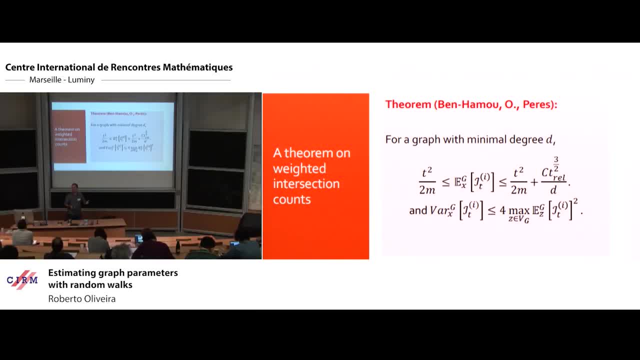 for the number of vertices, but what we just got is an estimate for the number of edges. for the same reasons before, And maybe I'm gonna write it over like I'm gonna fix this- I'm just gonna say if I wanna estimate the number of edges, 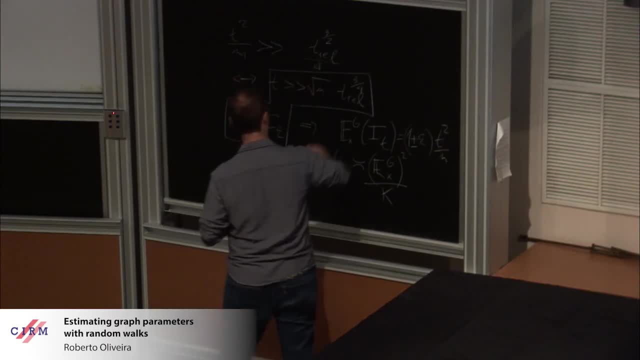 I need this to be greater than this, So I need something. yeah, maybe I'm missing a factor somewhere here. Okay, I know what the end result should be. Yeah, I think there is an error in the previous slide, because, oh no, no, that's right, that's correct. 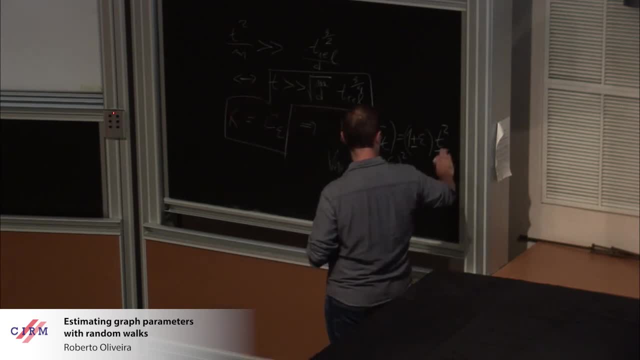 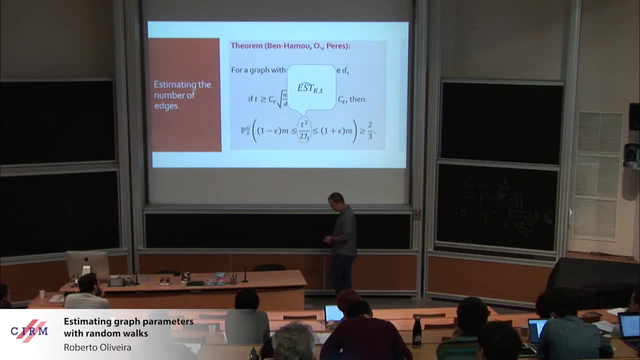 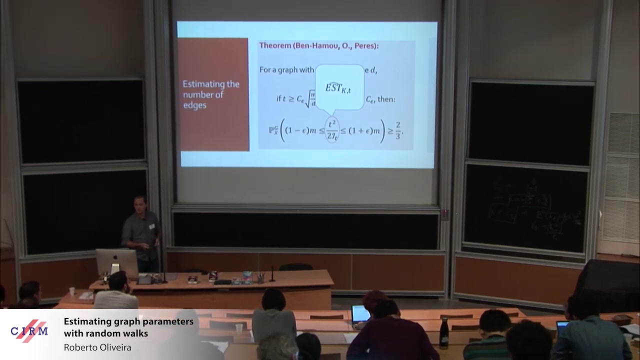 So I need this, And then I have this to be equal to two m and the variance is gonna be like the expectation squared. So now I mean basically, by doing a small modification of the previous estimator, I get an estimator for the number of edges. 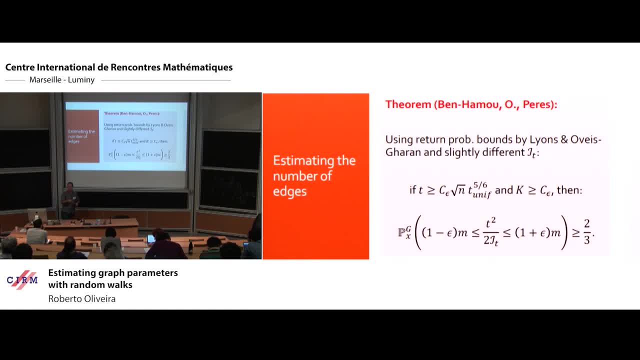 And there is another bound that you can use for these return probabilities. I mean, just write down the same calculation That was proved by Russell Lyons and Charles Hervéz-Garonne, which gives you another upper bound for the same quantity. 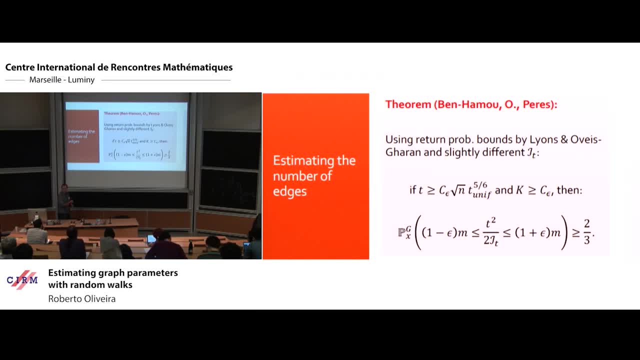 which now doesn't depend on the number of edges, depends on the number of vertices. But here you get the uniform mixing time raised to five over six. I mean, I'm not telling you what the bound is, but it's some bound of return probabilities. 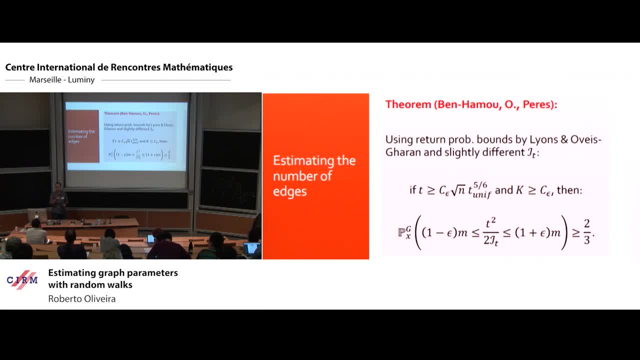 that's different from the one over square root of t bound that I showed you before. So this gives you another result on the time complexity for finding the number of edges, And I wanna quickly convince you that this- so you get an upper bound for t- well, k is always gonna be. 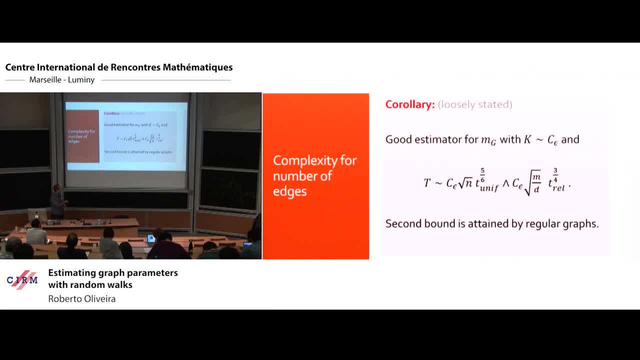 is always gonna be a constant in that case, and you get an upper bound for the optimal t which is like this: And I wanna convince you that this bound is sharp And okay. this is easy because for regular graphs, this is exactly what we had before, right? 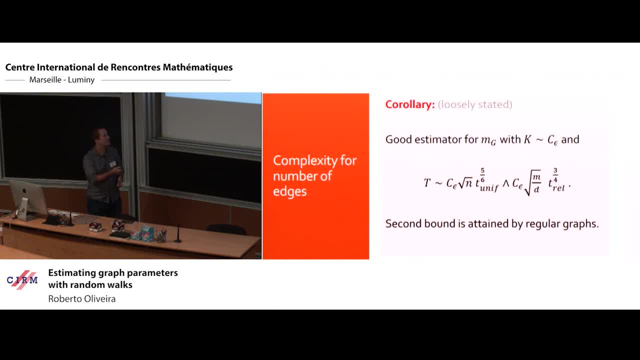 M is d times n over two, so this is n. What about this bound? How do I get a family of graphs for which this bound is tight? It's again based on this construction of expanders. So now, instead, remember that before. 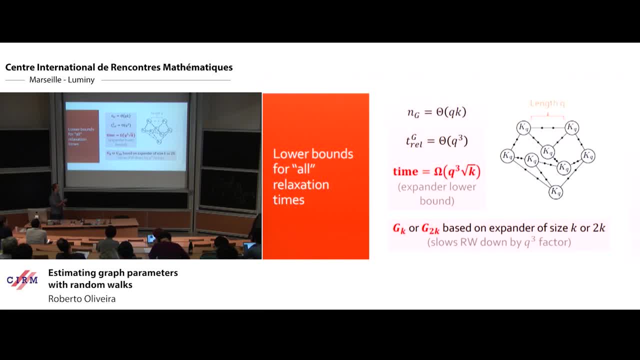 I subdivided the edges of the expander. Now, besides doing that, I'm gonna. so this is wrong. this should be length. no, this is right, sorry. So yeah, the kind of the letters don't really match. 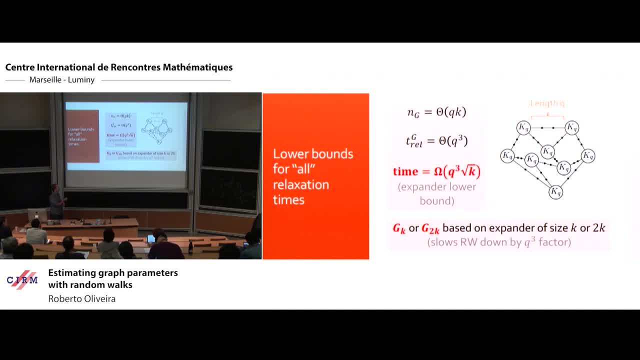 So this is an expander with k or two k vertices. I subdivide each path, each edge, into a path of length q and I replace each vertex with a clique right. So these edge I mean kind of. you know, I'm gonna pick three vertices. 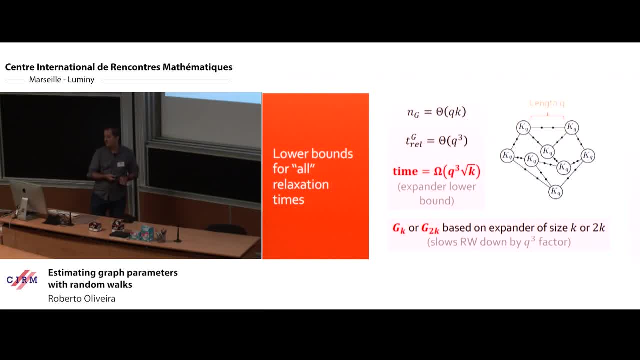 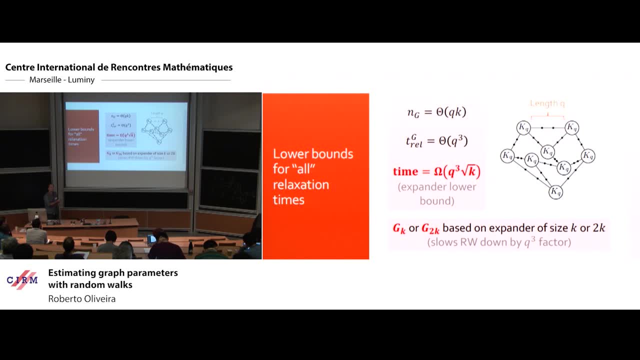 in the clique and connect them to these paths. And how long does it take for you to visit square root of k cliques, right, This is where the lower bound comes from. Well, basically, you have to- I mean you have to- look at the unit cost, say. 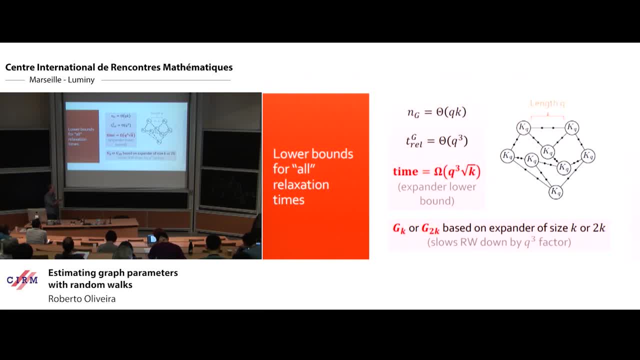 of crossing an edge in the expander right. What is it like? Okay, if I am lucky enough to reach a vertex from which I can cross a path, there's so much higher probability that it can come back Right. So if I come back to the clique, 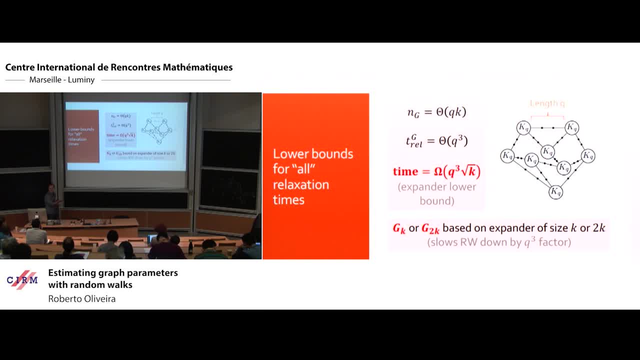 I'm gonna take time of the order of q to try to cross again. So on average I need q squared steps to cross the edge, but I'll need q attempts to do that. So I slow down by a factor of q to the cube. 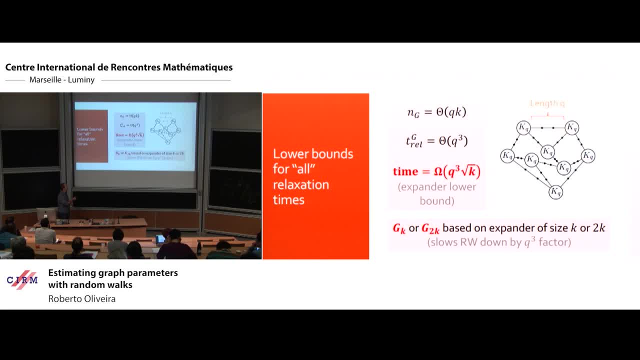 And that requires some thought, but that's basically the idea. You need q squared time to cross once, but you need lots of attempts to actually do it, And so the relaxation time's like q cubed, And then the time it takes you. 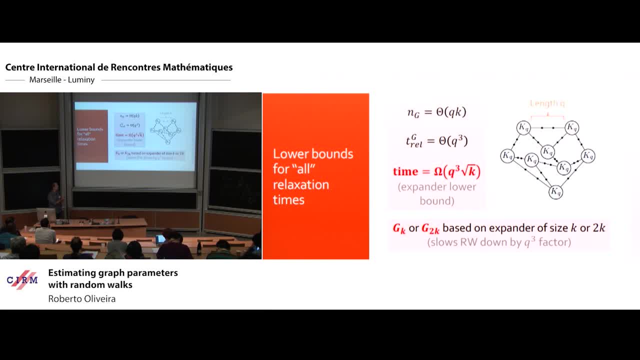 again it's like before. right, The square root of k comes from the expander bound and q cubed. is this extra factor that you get And you work it out and it turns out this gives exactly this number right. 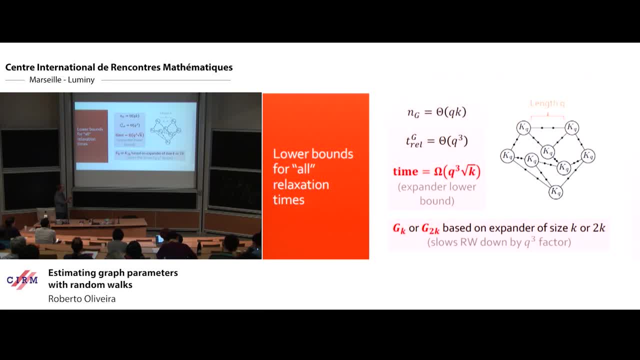 So you can see it right. So if you put a q in here, you get q raised to five halves and that's the relaxation time raised to five over six. So oddly enough, this very kind of weird-looking bound is also tight. 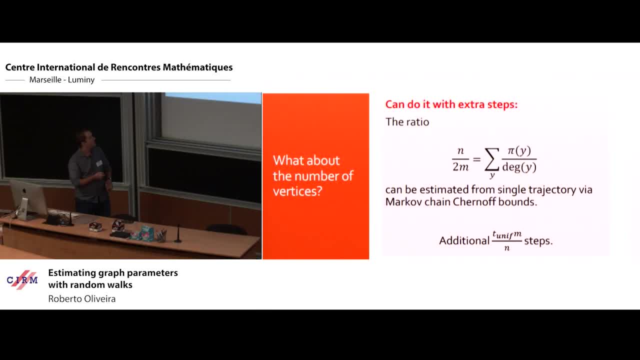 Right, so let me just say something. Okay, once you can estimate the number of vertices, you can estimate the number of sorry. once you can estimate the number of edges, you can estimate the number of vertices by computing the average degree. 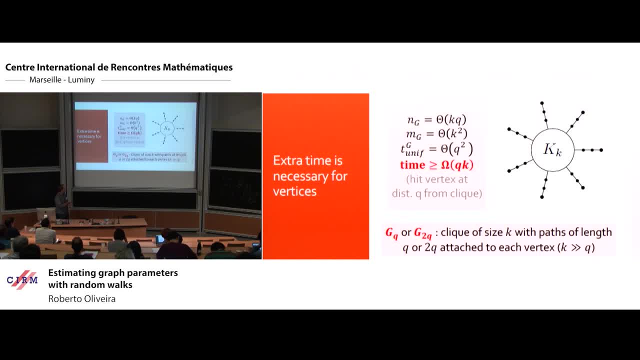 This you can do in this time and perhaps I don't have time to explain, but there is a. I mean, you really need additional time to estimate the number of vertices, right, And the additional time you need is this thing here. 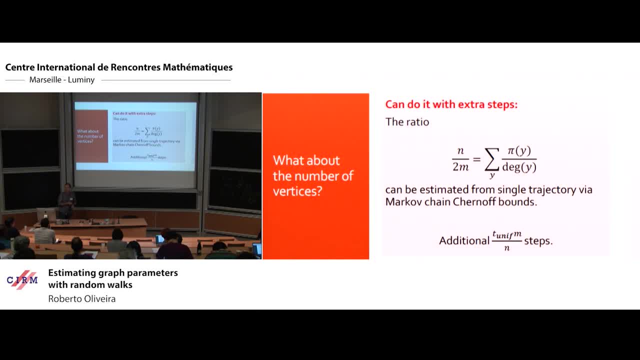 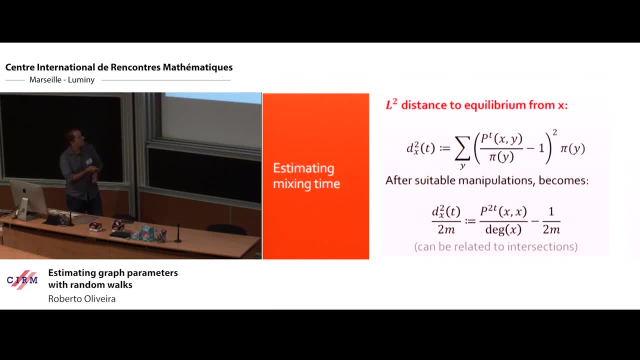 Up to log factors, assuming if m divided by n, And there is some example to prove that, And so this is a bound you need for the number of vertices. Let me quickly say that if you wanna compute the L to distance, to equilibrium, right. 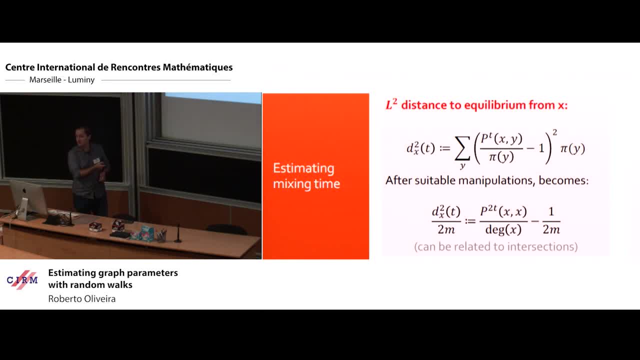 so notion of mixing from the specific vertex x, as we know, we can also relate that to return probabilities And once you know that, you can also devise an estimator for the mixing time from the same ideas, right. So return probabilities, as we saw, 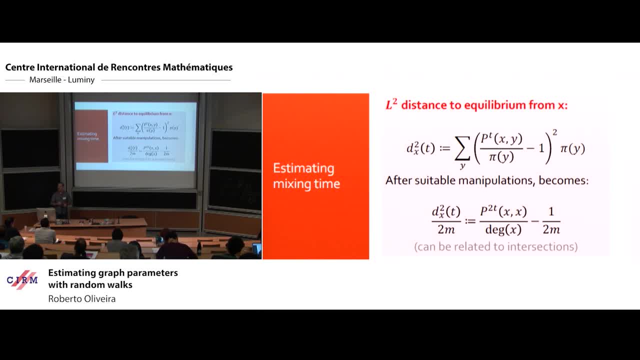 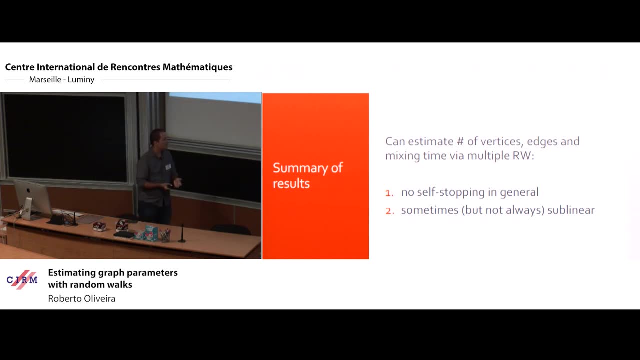 are related to intersection probabilities of paths. And then if we can devise an estimator based on intersections for the mixing time And okay, so what do we see? We saw that basically, by looking at random walk intersections, we can get optimal estimators for these three parameters. 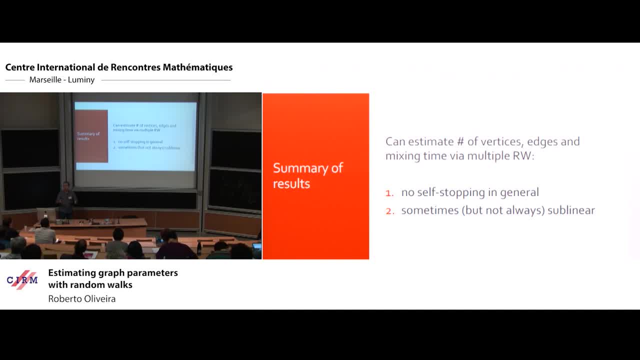 number of vertices, number of edges and the mixing time from a specific vertex. And. but we also saw there are limitations, right? So I mean there are no self-stopping algorithms of this kind that decides on its own when to stop. 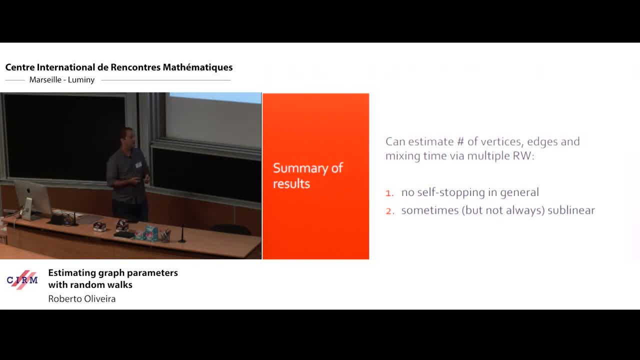 And they're not gonna be sub-linear algorithms. in general, You really need a small relaxation time or mixing time for that to work, But of course there are many open problems, right, Because you can ask about other graph parameters. how do you estimate anything else about the graph? 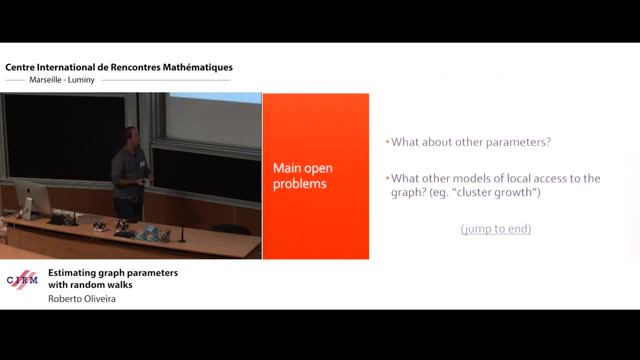 We don't really know. And there's some other thing which is that okay. somehow, the way I try to convince you that this is a reasonable model for computation, say, well, it's easy to implement. well, people actually implement random walks in real life. 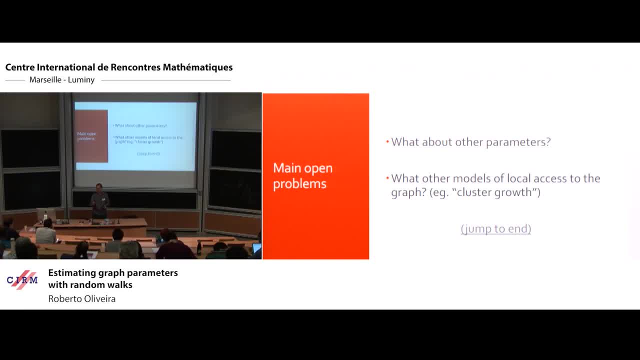 right. so, but the way they do it is basically. I mean, the way random walks are nice is that you're using this algorithm where you just explore the graph little by little and you just need to walk from vertices. you've seen to neighbors of those vertices, right? 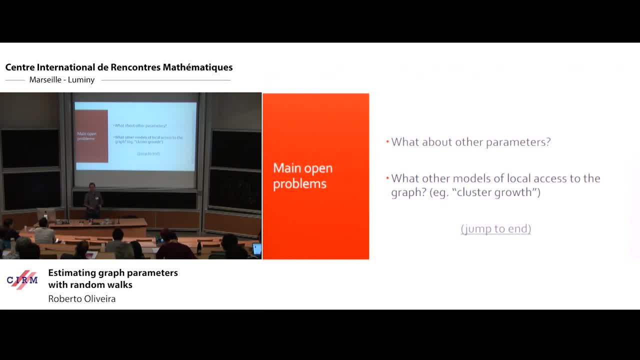 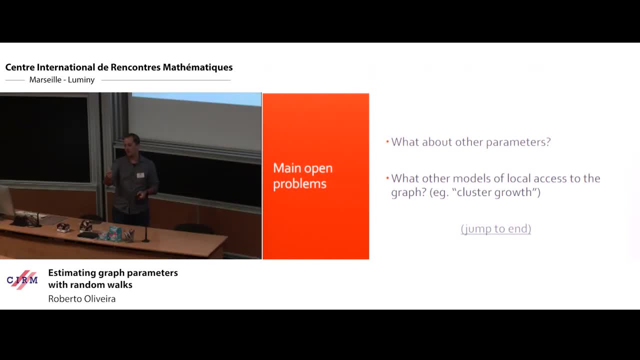 So there's a more general class of algorithms that you could think. that's like that. Perhaps you have a set of vertices- right, The vertices you have seen and you know their degrees, and you can ask to see a neighbor, a new vertex at the boundary of the set. 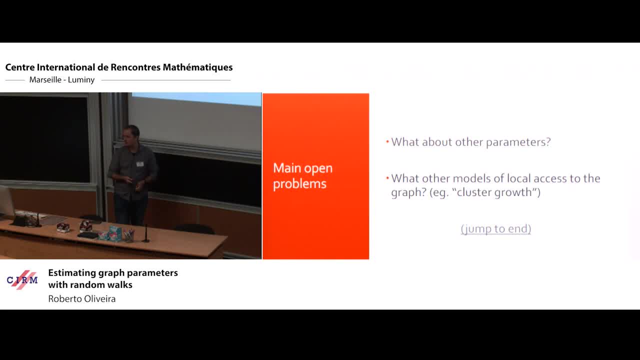 perhaps picked at random somehow. I talked about that before. as I said, the expander lower bound also works for this model, where you just query the graph little by little, But we don't know. I mean so for expanders. 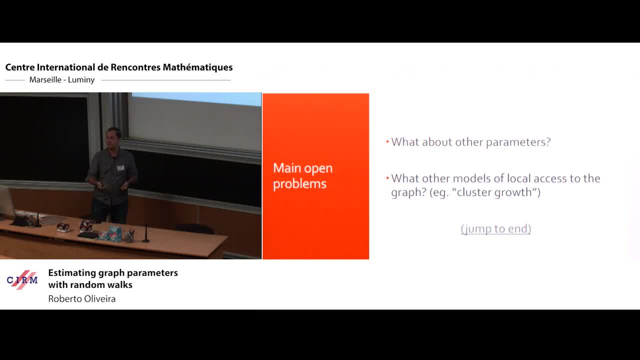 in some sense random walk intersections are optimal, even if you're allowed for a more general model, but we don't know that that's true for more general things and actually there are lower bound examples that are based on the fact that it takes you a long time. 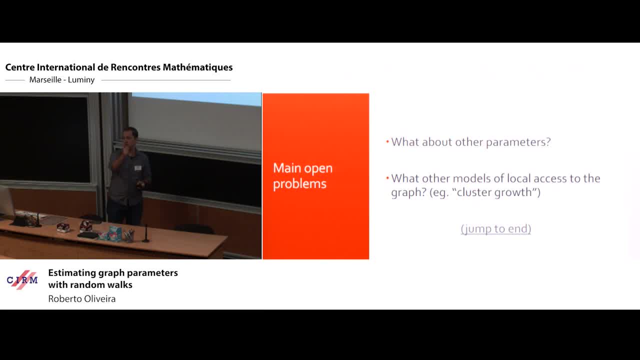 to cross a path, which is not gonna be true in this model. You can basically just move forward on the path. So what's the right parameter to study this model? I venture to guess that it's the Cheega constant, but it's an open problem.